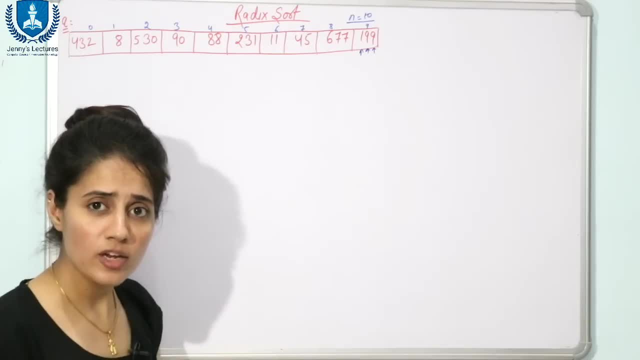 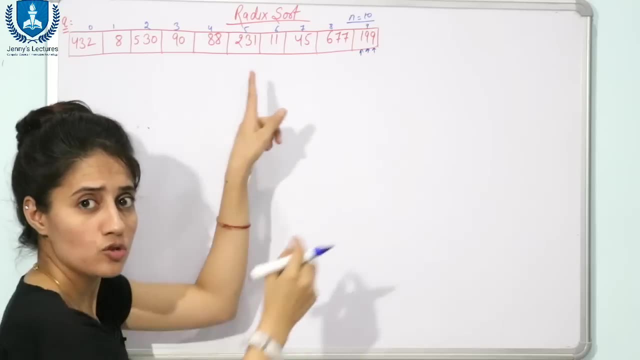 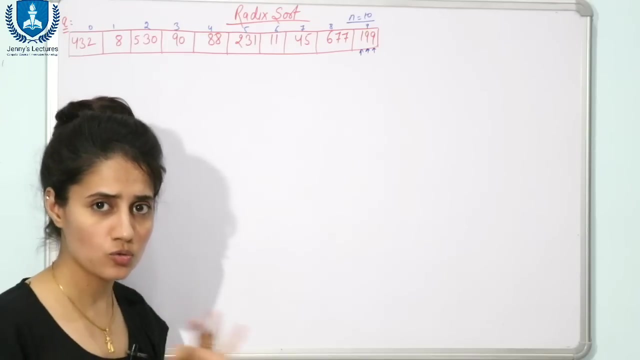 be sorted. if numbers are given, if in the strings values are given, names are given, in that case you apply from msb to lsb. but in case of integers or numbers you are going to apply from lsb to msb. in this direction we are going to apply counting sort. fine. so first of all, how many? 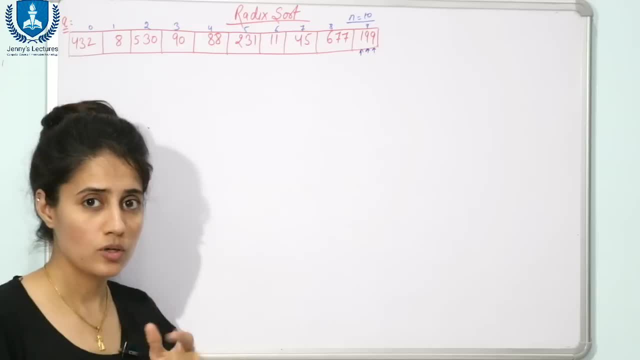 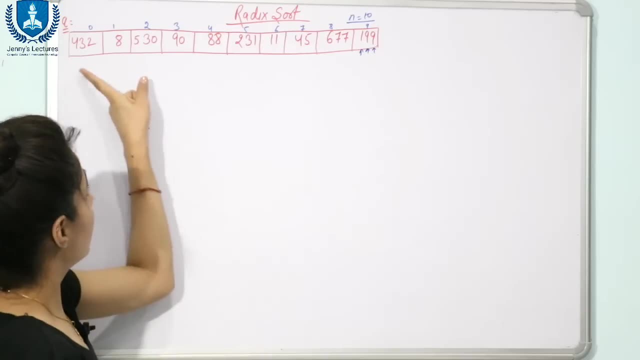 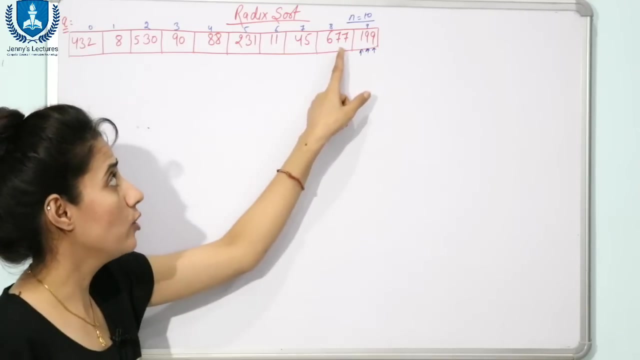 how many times counting sort would be applied that you have to count so out of given array. first thing is you have to find out the maximum data in this area. the maximum data is what? 677.. and count how many digits are there in the maximum data? one, two and three digits. so how many? 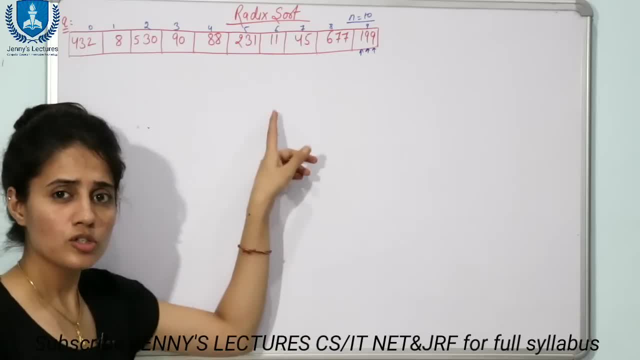 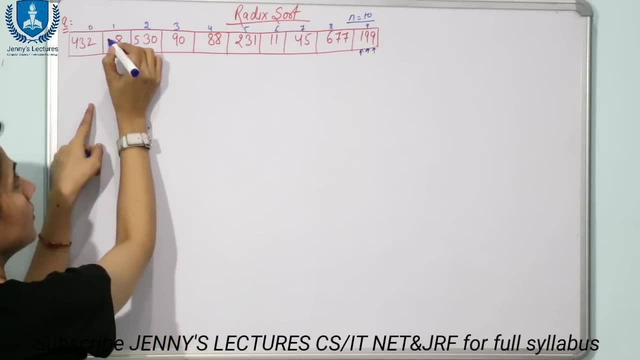 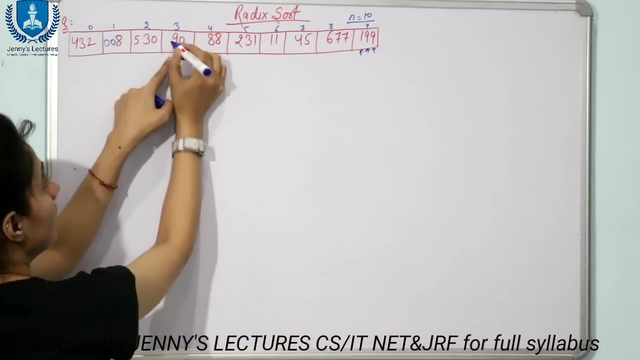 times, counting sort would be applied three times. now we are supposed to make all the numbers three digit numbers, so this is eight. how you can make it a three digit number? just add two zeros to the this side, fine, not to the right hand side, to the left hand side. here one zero. here one zero here. 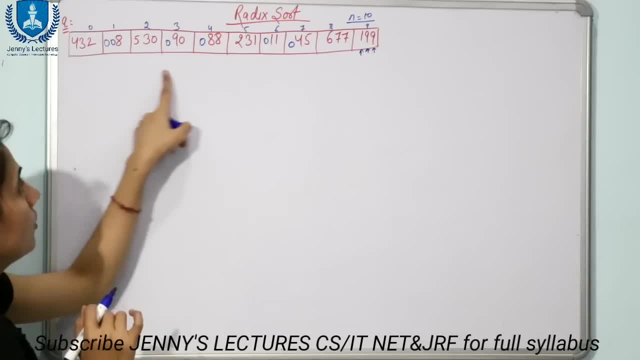 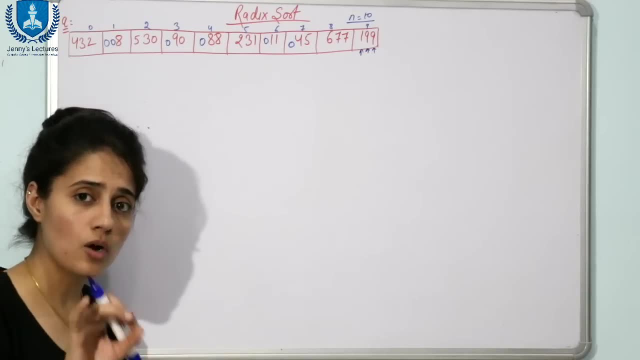 we have one zero here. we have one zero. now, all we have to do is we have to make all the numbers. all the numbers are three digit numbers. now we are done with our first step. now next step is what you are supposed to apply now: the counting sort. now i'm going to show you how actually count sort. 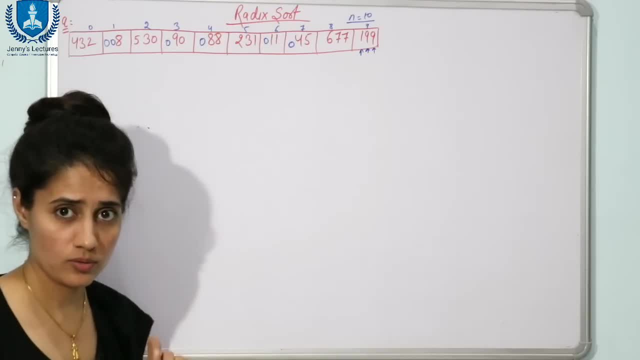 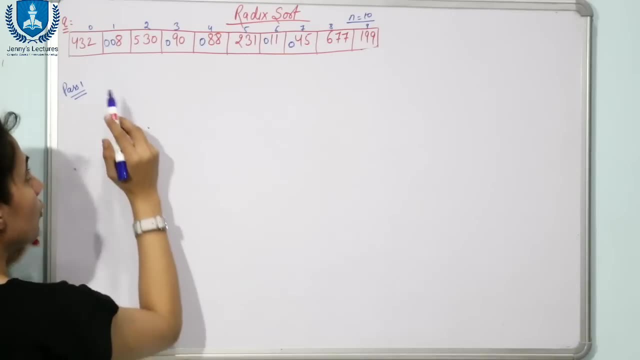 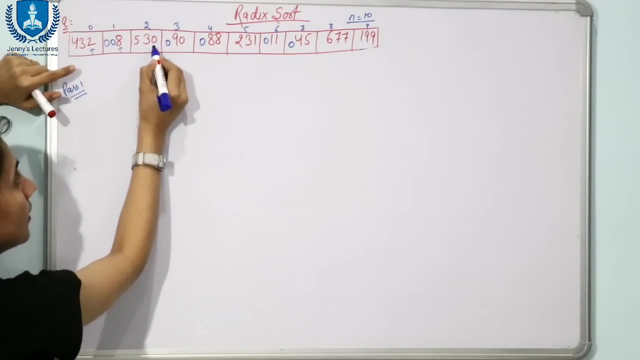 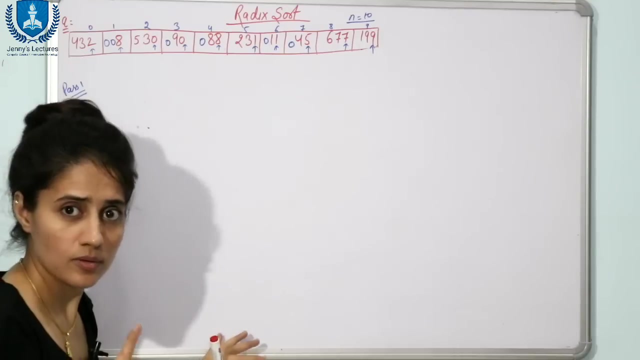 would be applied in redix sort. so three passes would be there. now, first pass in, first pass you are going to apply count sort in on this place value, on the ones place here. you can say, here, here, on these key values, on the least significant bit, we are going to apply the count sort. fine, now see. 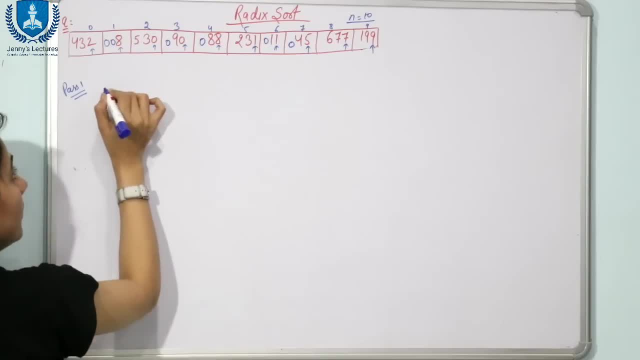 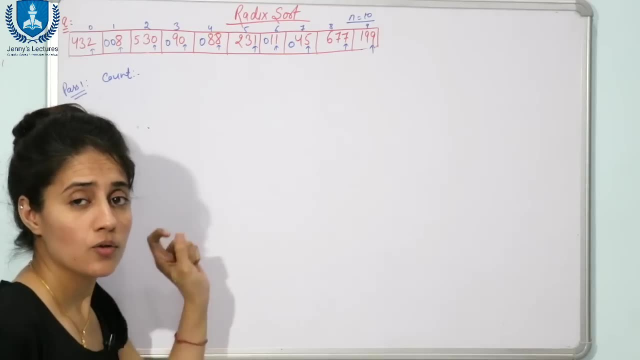 what is the procedure to apply count sort? we are going to take one count array and the size of this count array would be see in redix sort. the what is the k value range is from 0 to 9 because the c each digit would be. 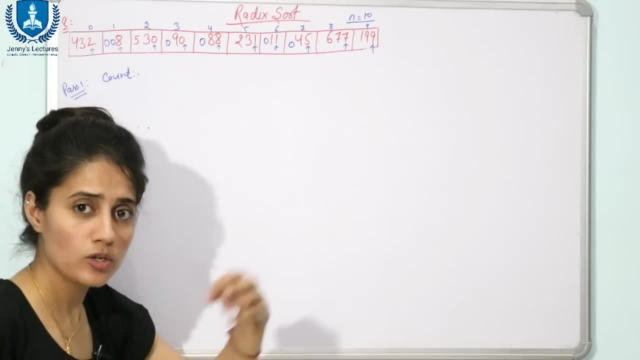 either 0, 1 or 2 or up to 9.. so you are, you are going to take the range 0 to 9.. so k value is 9.. so the size of this count array is what? 10.. so this is our count array: size is 10. and first of, 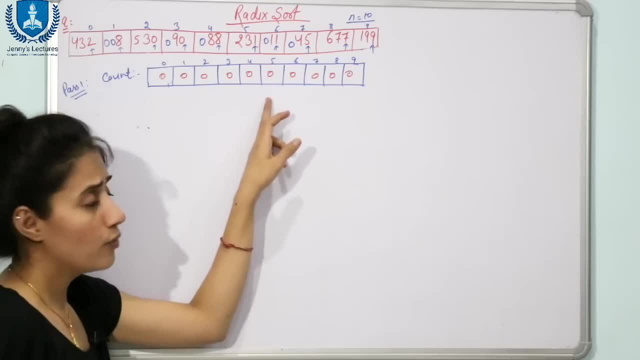 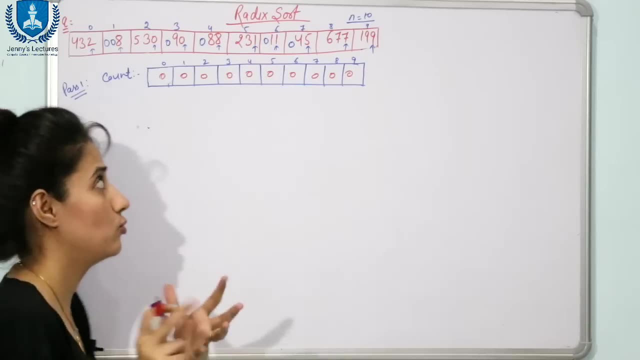 all, we are going to initialize this array with 0.. now what you are going to fill in this area? we are going to count the count, the elements, the frequency of the elements, according to the distinct key values. fine, that i have discussed in count. so that is why i am again and again saying: please watch. 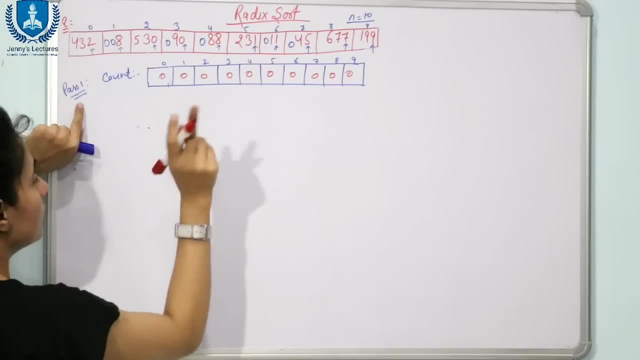 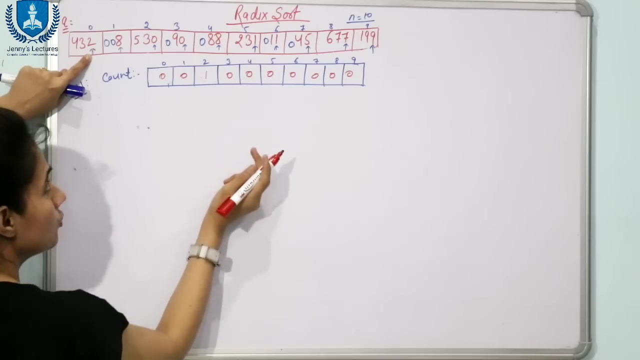 that video first of all. so here counting sort would be applied in first pass on this digit on the index, because this count array is a significant digit. so check out this digit. here we have 2. fine, so here we have 2. then go to the index 2 and increment this counter. that is 1. next we are. 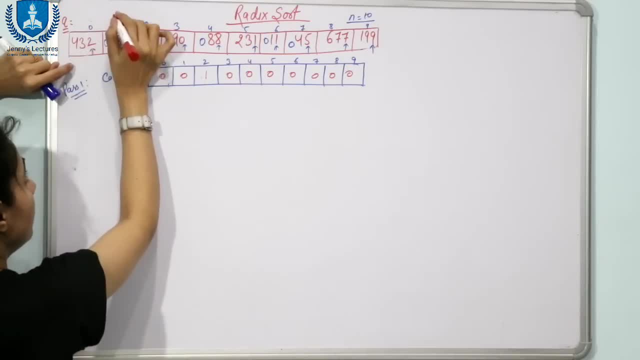 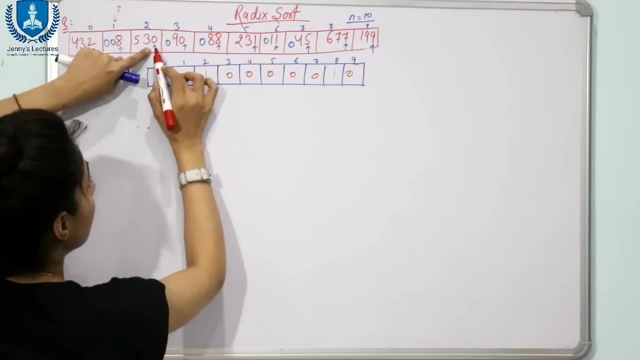 going to take first that variable i, and we are going to start a loop now. i value would be incremented. here we have i and check out this digit. here we have 8. so go to the index 8 and increment this value. here we have 0. go to the index 0 and increment this value. 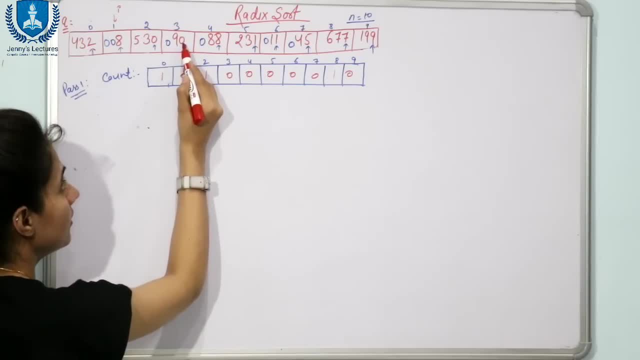 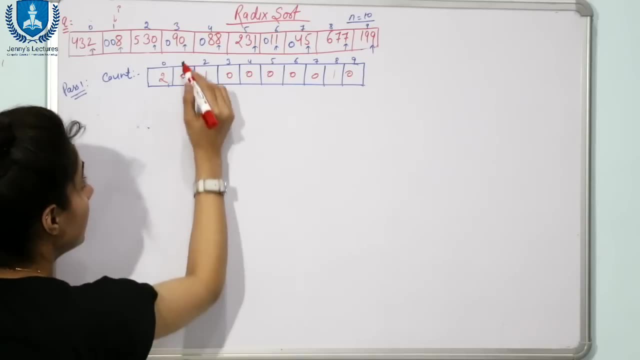 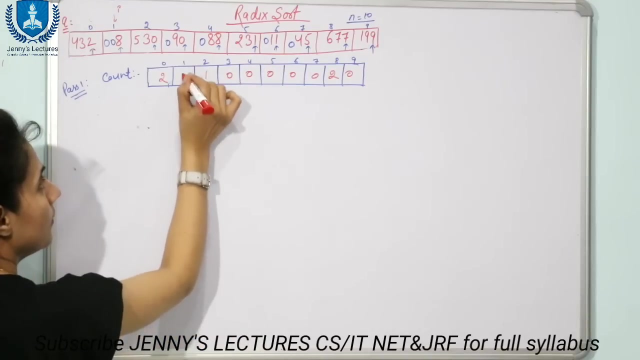 we have 0 on the least significant digit, or you can say at the ones place. so again, go to index 0 and increment this count value. fine, here we have 8. go to the 8th index, increment this value. here we have 1. go to the index 1, increment this value again 1. increment this value 5. increment value at. 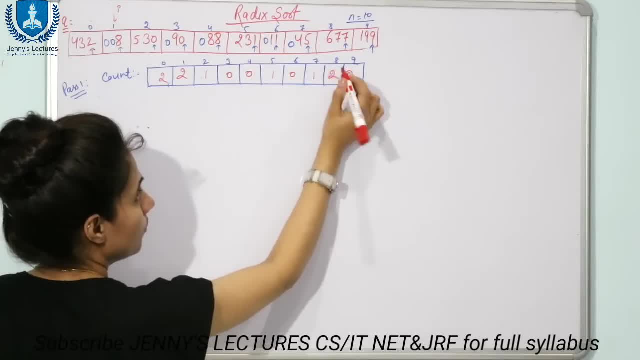 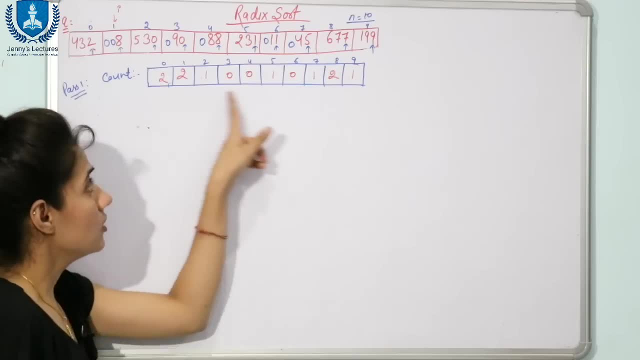 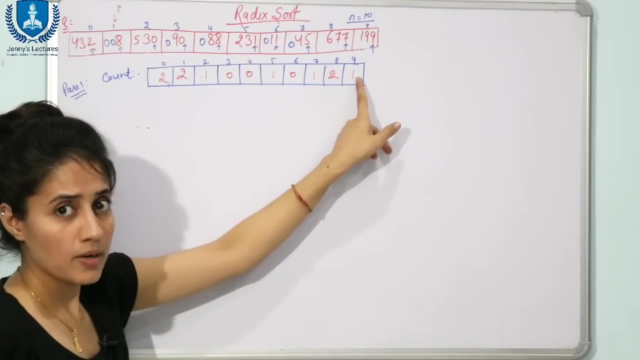 index 5. 7. go to index 7: increment this value. 9: go to index 9: increment this value. that is done now. this is our count array. we know now see, in this case 9 is only one time at the ones place only, because now we are applying the count sort on the one digit only. 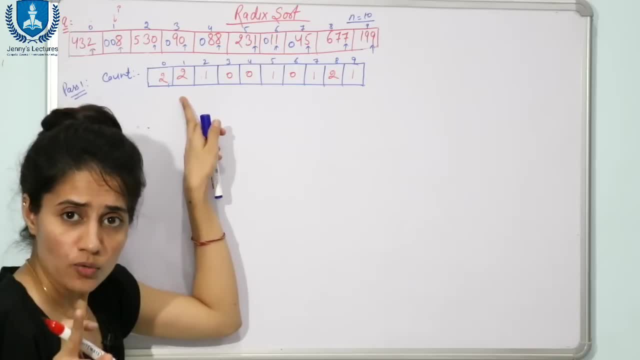 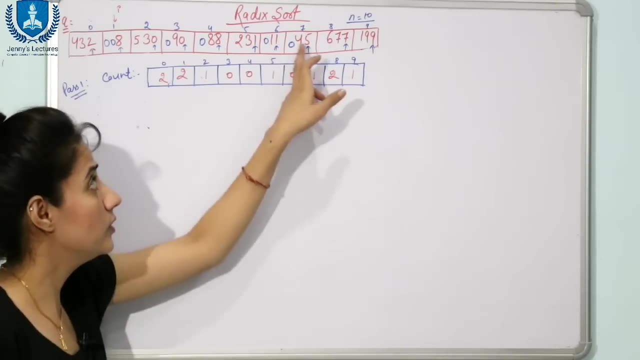 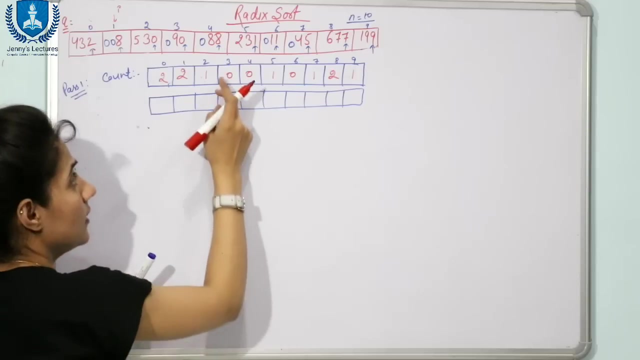 fine, now you are going to update this count array. second step was: we are going to update this count array and such that this count array would contains the actual position of these elements in the sorted array. fine, so how to update this count array? see, we are going to update this count array only. 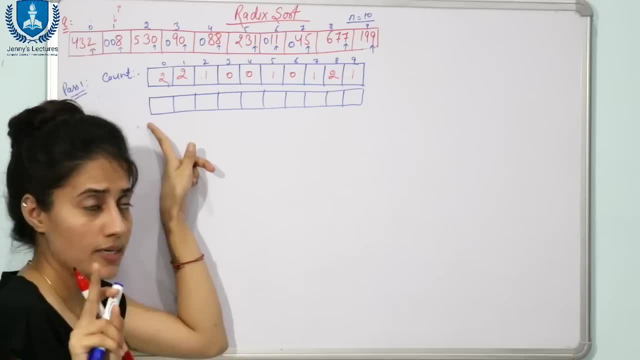 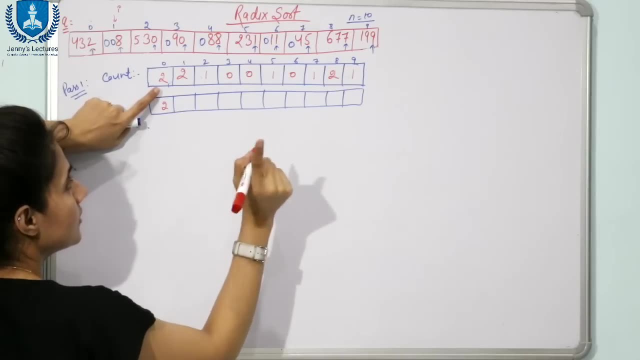 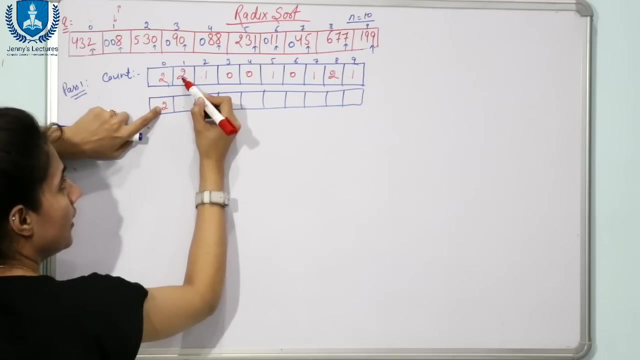 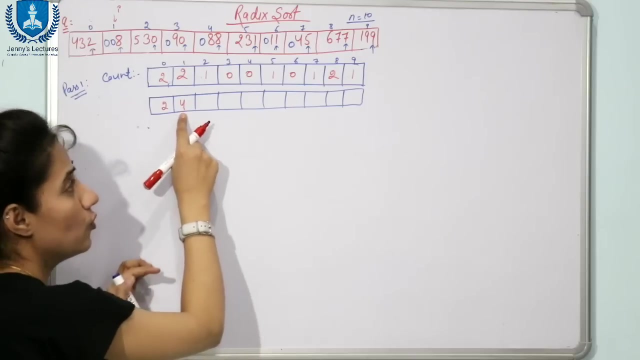 fine, i am just making another array just for the understanding purpose. so see first what is the? what is the step? first value would be as it is now. next step, next step would be how to fill this value. here is we have 2 and the next value is 2, so 2 plus 2 is 4. fine, at position 4. or you can say: 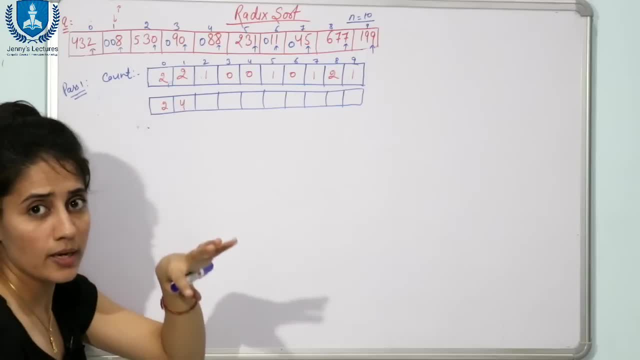 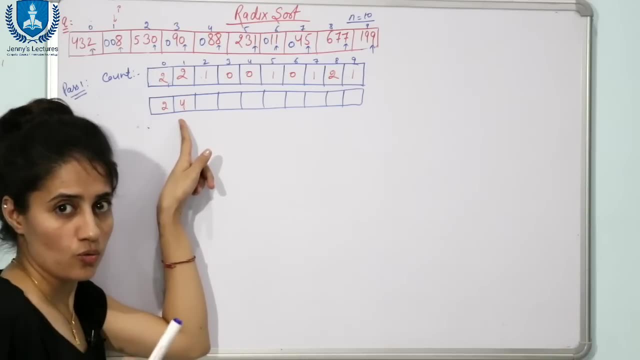 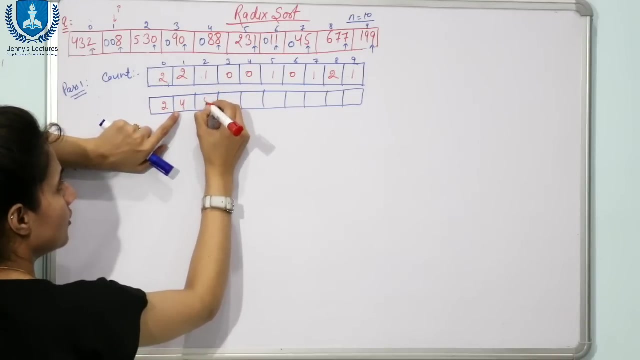 index 3 till index 3: 1 would be there in the sorted array. fine, see this. this fund. i have clearly explained when i was explaining count so fine, so please check out that video now. we are going to add 4 plus 1, that is 5. 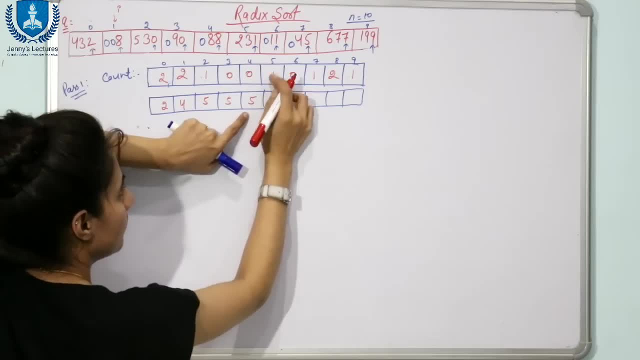 5 plus 0 is 5, 5 plus 0 is 5, 5 plus 1 is 6, 6 plus 0 is 6, 6 plus 1 is 7, 7, 9, 9 plus 1 is 10. 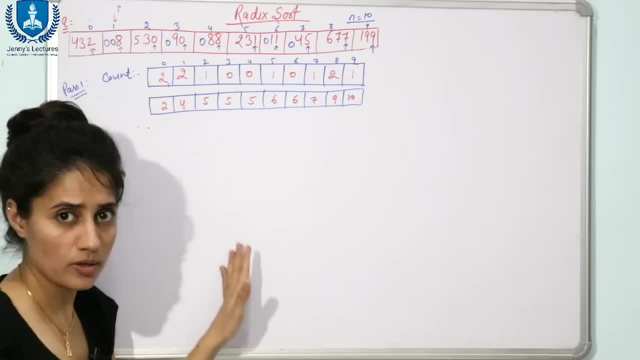 fine, so this is the actual position of these elements in the sorted, when you are going to find out the sorted array now. now, what you will do: now we are going to build the output array. fine, we are going to sort these elements according to one digit only, that is, according to this digit. 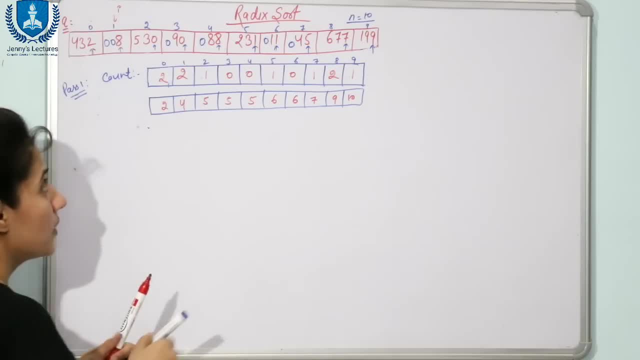 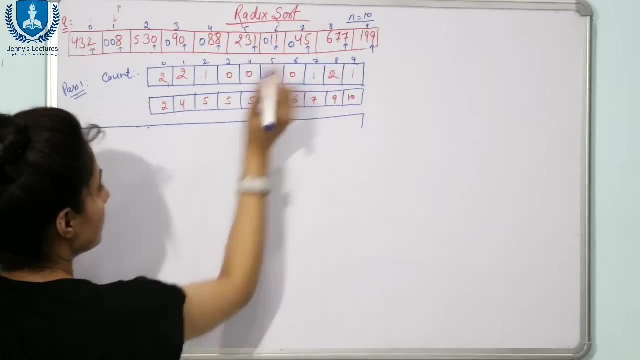 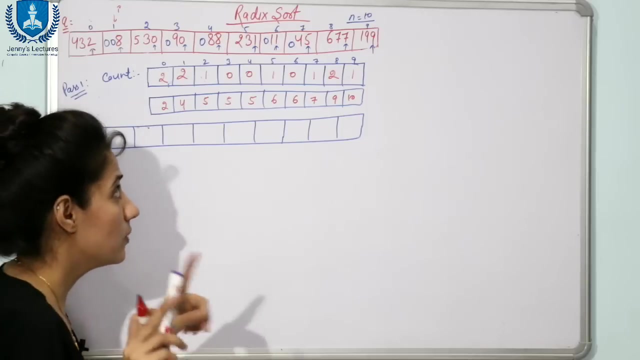 only first of all now go. you are going to build a array. now take another array. suppose i am going to take an array b, and that array would be same as size array a, the original array given. so now this is array b. how to build this array? what was the processor? see, we are going to scan this array from right to left. 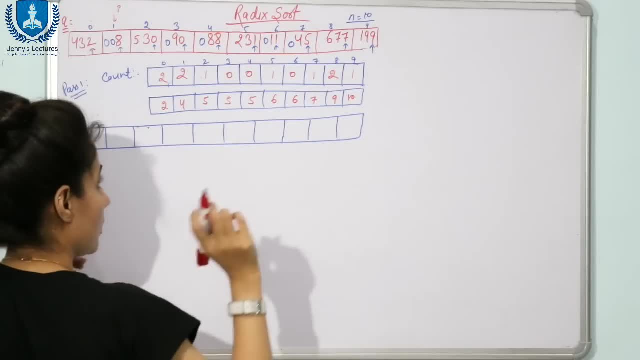 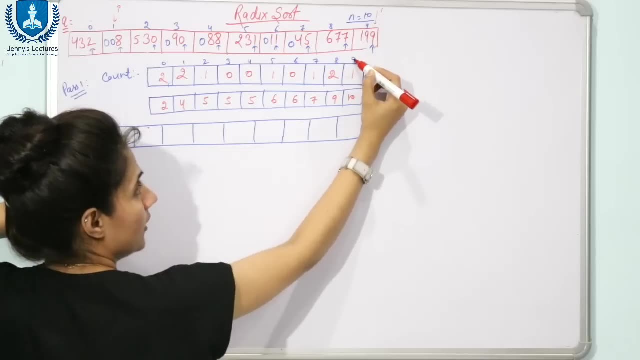 why this? because to maintain the stability property of this counting sort here, scan this. here we have, suppose, i, the element at this place is 9 and we are going to scan this array from right to left. so we are going to look at the index. so now we are going to commit the i to the index. 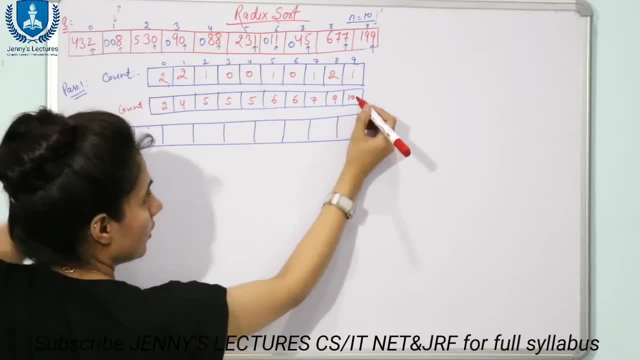 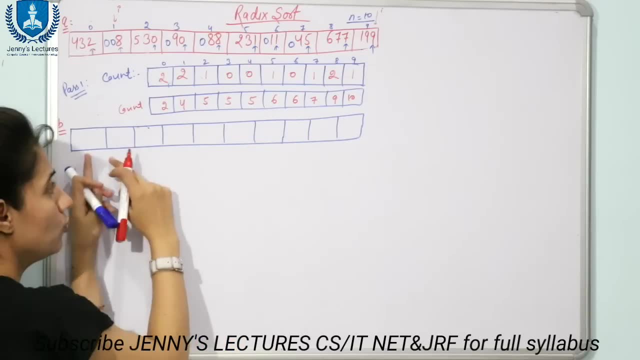 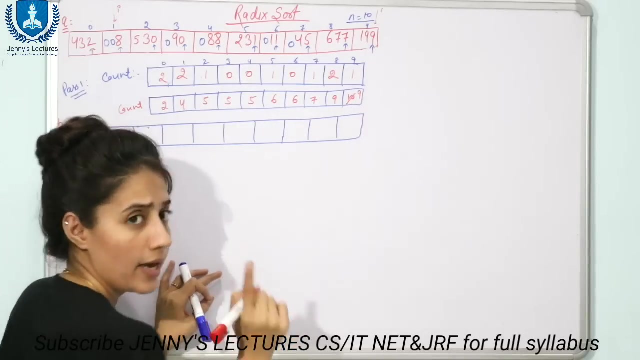 it is 9. so go to the index 9 in count array and the value is 10. see, this is the updated count array. we are going to check this one. we are not going to check this. one value is 10, but this is count fine, and we are going to apply. we are going to work with work with the indexes. so, first of all, 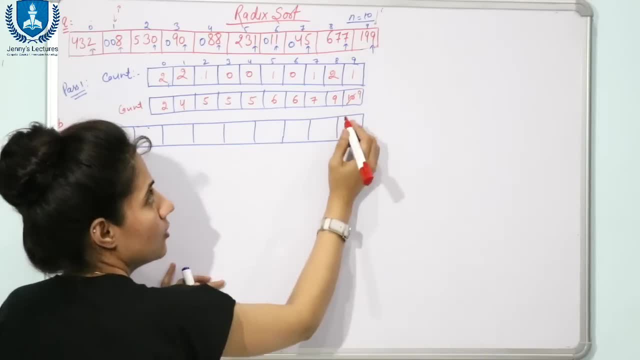 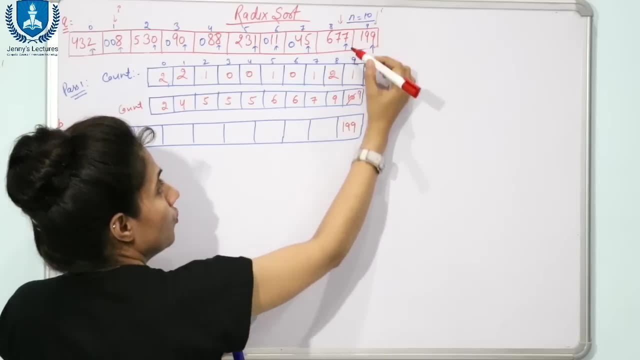 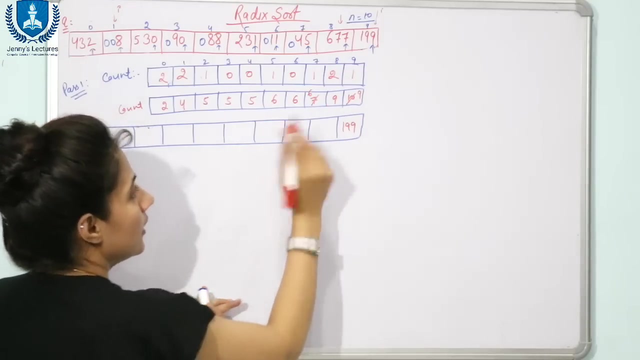 we will decrease this 10 minus 1, that is 9. here you will put 199. this is index 9. fine, now decrement. i value check out this number. key value 7: go to the index 7. value is 7. first decrement this value, that is 6. now go to the index 6 and. 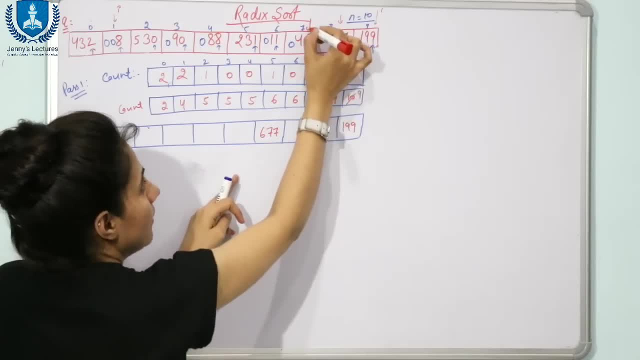 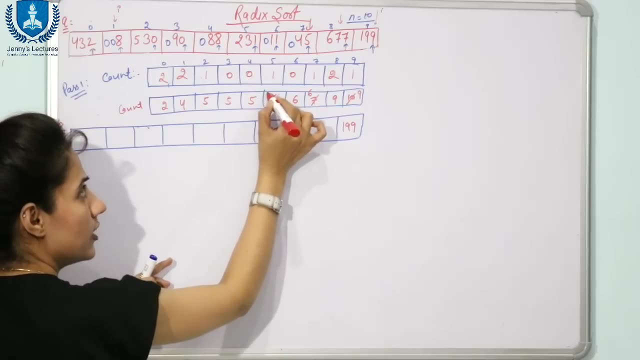 place this value: 677. decrement again i value. here we have 5. go to the index 5. here we have 6. decrement this: first of all. that is 5. go to index this 5. this is index 5. next is 1. go to the index. 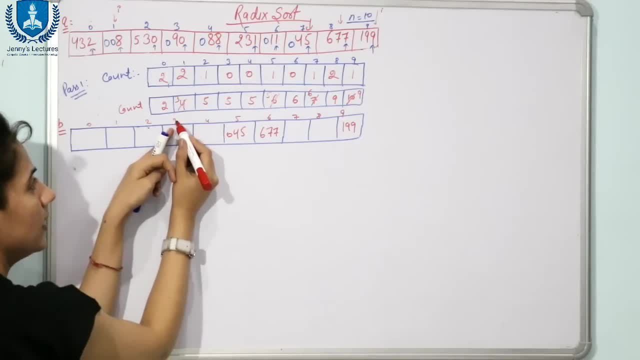 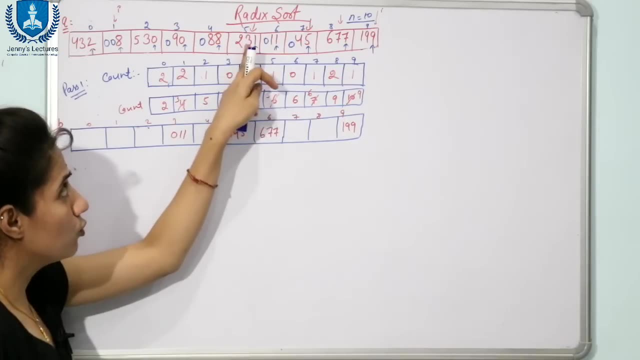 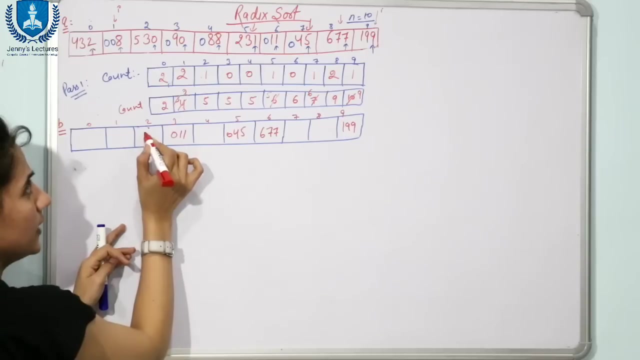 1. here is we have 4. decrement this value at index 3 in this output array. place this value 011 again decrement i: we have 231. value is 1. go to the index 1. decrement this value, that is 2. on second index you are going to store 231. now decrement i: here we have 8. 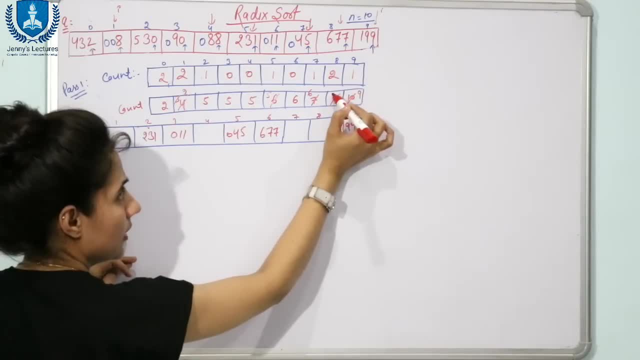 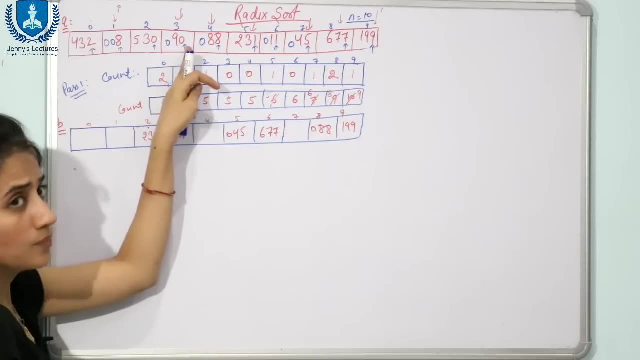 at once place. go to the index 8. here we have 9. decrement this, first of all 8. at 8th index you will store 88. now again decrement i. here we have 0. go to the 0th index. here we have 2 count. 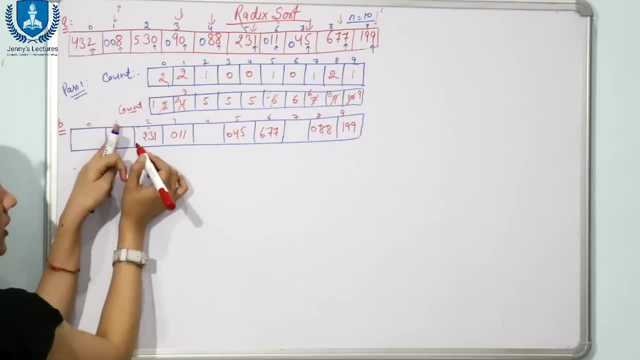 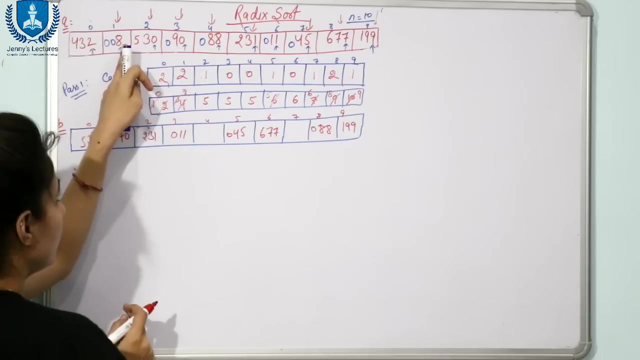 value is 2 decrement this, that is 1 in index 1 in the output array. place this value. that is 90 decrement i value 530 means we have 0 here. go to the index 0 decrement this value. that is 0. at 0th index you will store what 530 decrement i value 8. we have 8 now at once place. go to the. 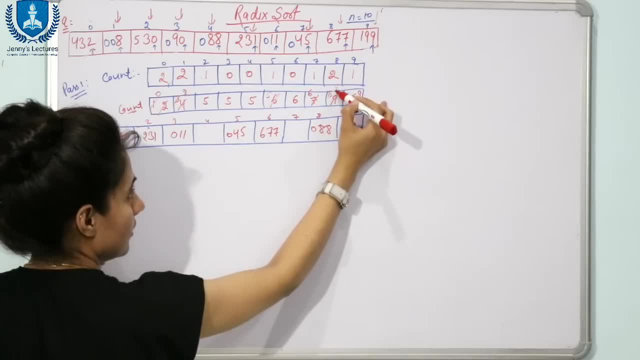 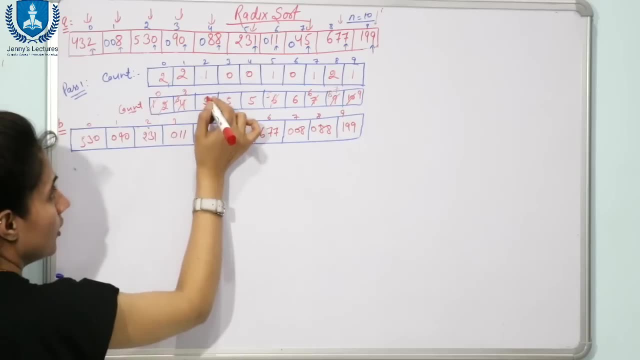 index 8 value is 8 decrement this. that is 7 at 7. you are going to place this 8 now this value 2 go to the index 2. here we have 5 decrement this 4. here you will put 432. now we are going to store. 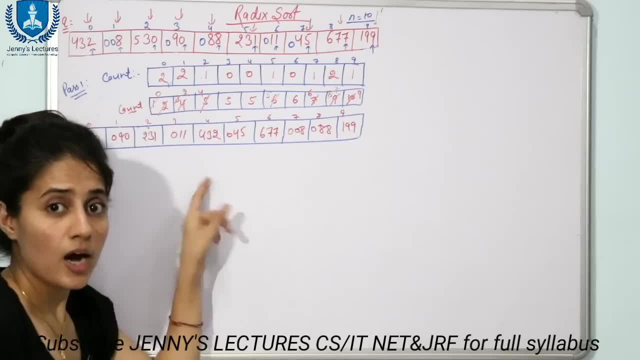 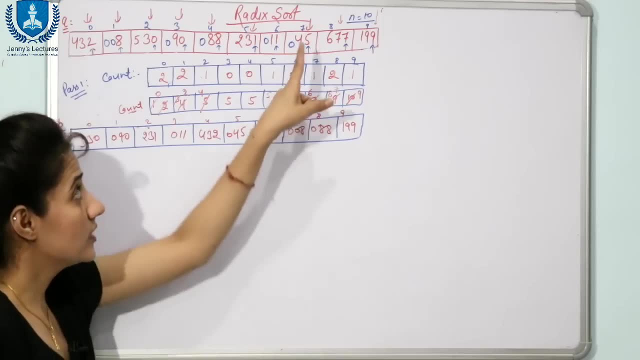 because we have raised to index 0.. Now this is our array after pass 1. see, we have just sorted the array. we have applied the count sort on only one digit. we are still remaining with two digits. so this is now the array. now, now we are. 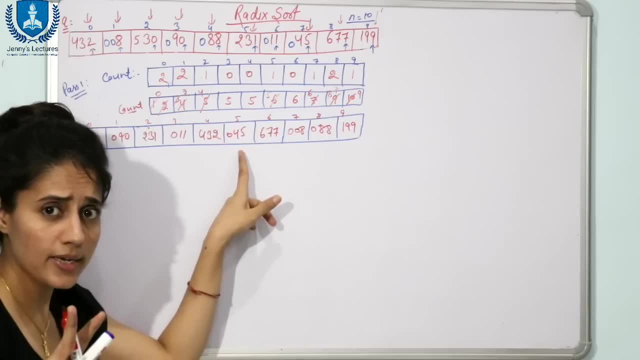 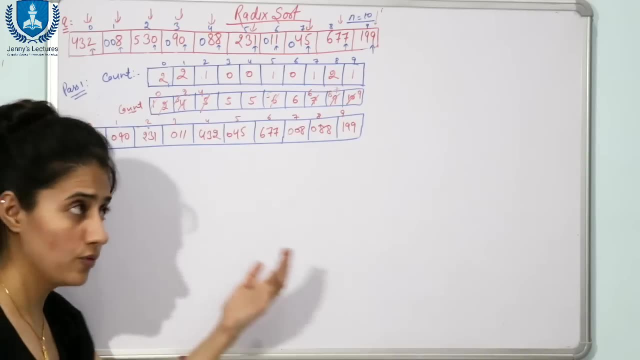 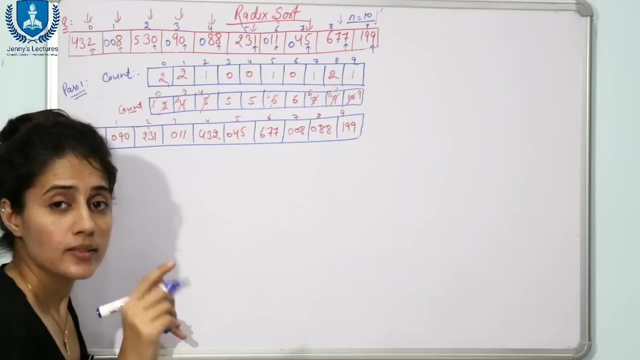 going to apply. this is now your array, updated array. what you can do, you can just copy these elements into this array with applying a one for loop. fine, now, this is our updated array. now we are going to apply the count. sort again: on which digit digit, the digit which is at tense place here. this one, second, this one. 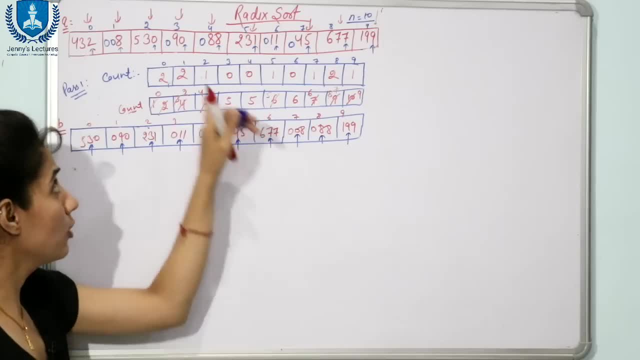 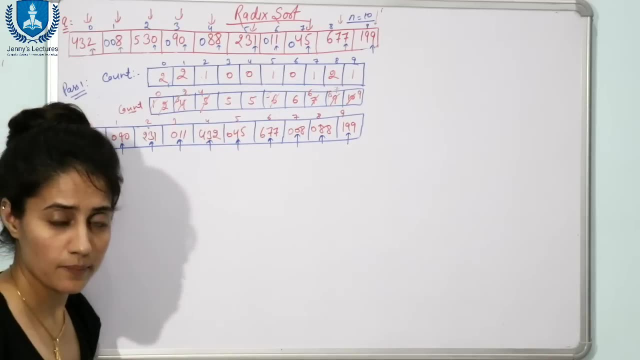 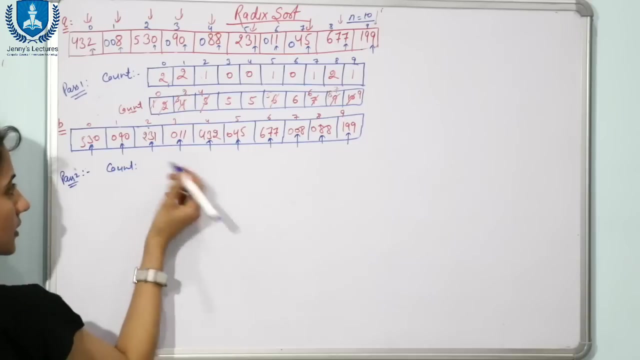 same procedure would be followed for this digit: same, you are going to uh, build this count array. same, you are going to fill this array. and now, again, you are going to build the output array. fine, so this is pass 2. now, same, we are going to take the count array. 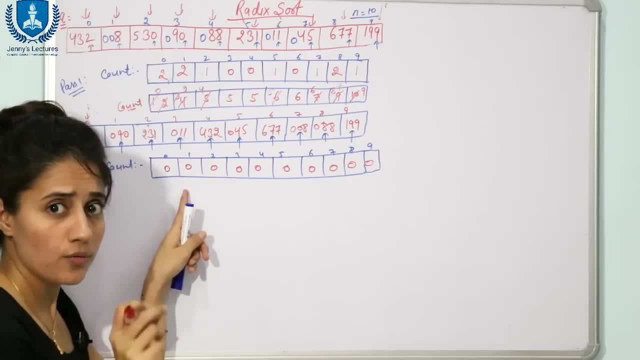 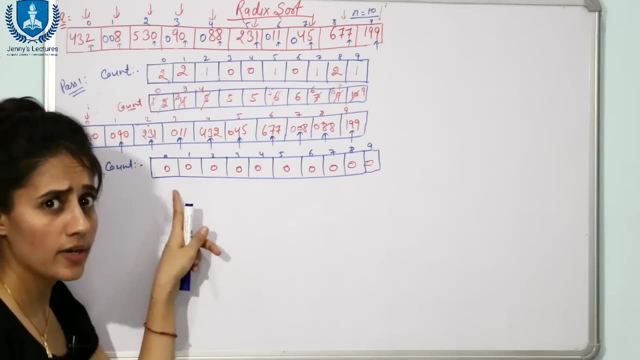 count array: again, we are going to initialize this count array with values zero. fine, see, we are going to update the same array. it's not like: here counter is different, here counter is different. the same array you are going to take in the program. i am just drawing this error again and again. fine, 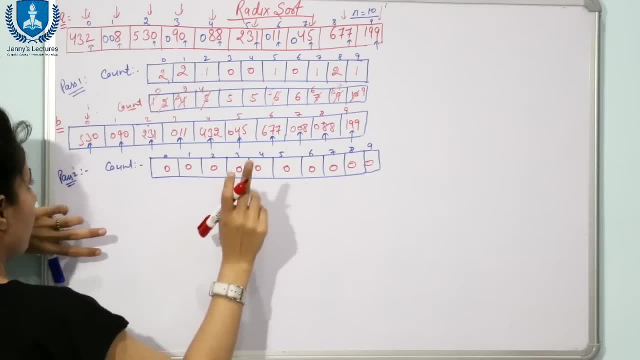 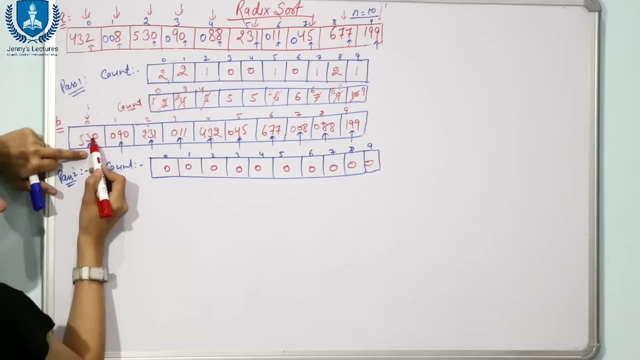 see now how to fill this area. we are just, we will counter the frequency of the element. see now, i would be started from here. now we are going to apply count sort on this digit, digit at tens place. now here we have three. go to the index, three in the counter and increment. 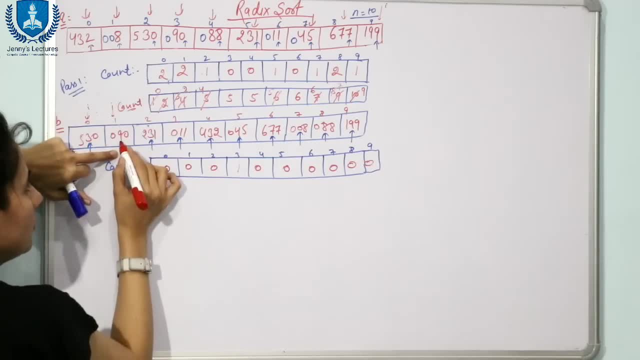 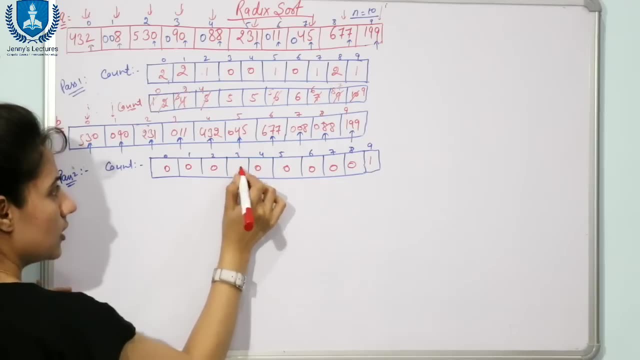 this value. next increment i. here we have nine. go to the index nine. increment this value. here we have three. increment at index three. increment this value. go to index three and increment this value. next we have one. go to index one. increment this value. next is three. go to the index three. 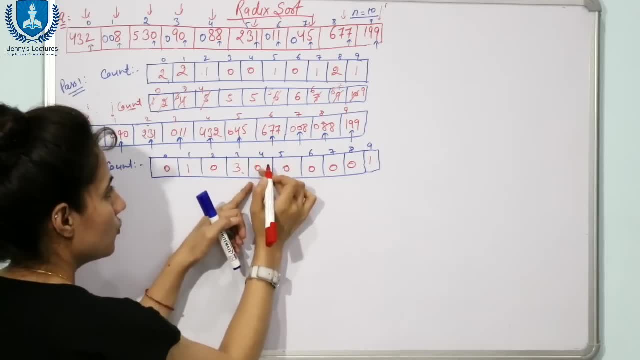 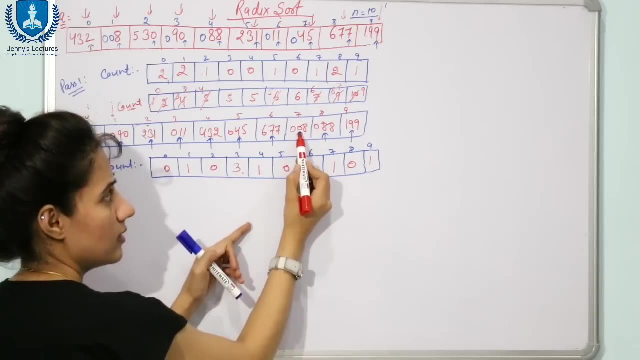 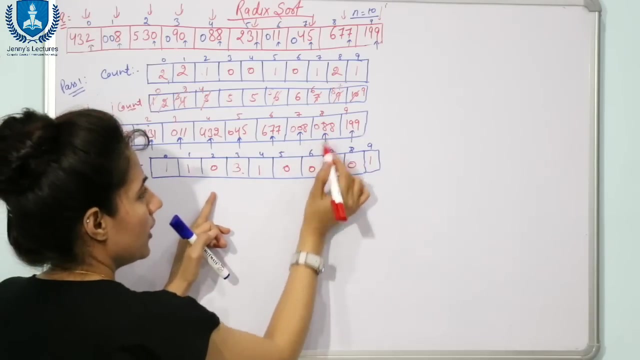 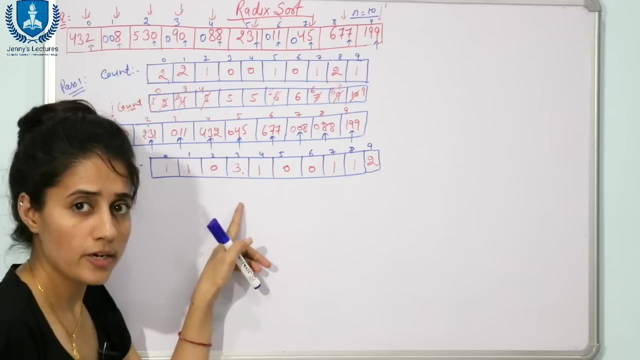 increment this value. next is four: go to index four. increment this value. next is seven: go to index seven. increment this value. next is see second desert. here is zero, fine, so go to index zero. increment this value. here we have eight: go to index eight. increment this value. here we have nine: go to index nine. increment this value now. this is our counter. 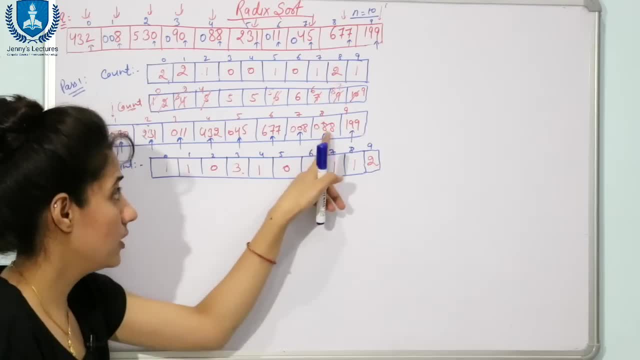 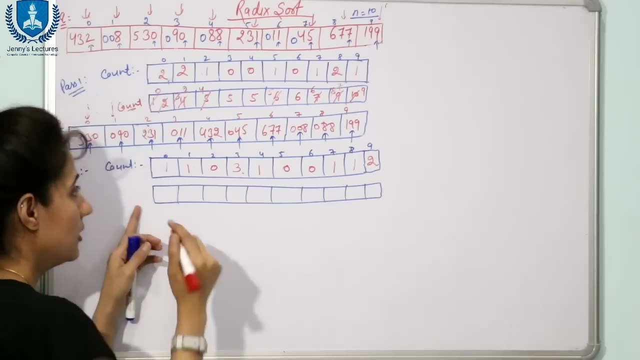 and now we are going to update this counter array to reflect the actual position of these, these numbers or elements, in the sorted array. now how we are going to update this counter, same would be followed. first value would be, as it is, the value at 0th index. we are going to start the 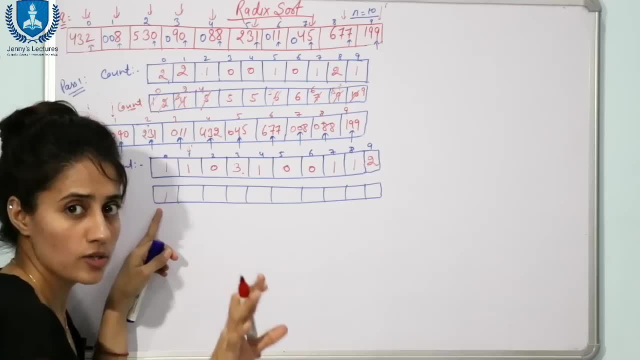 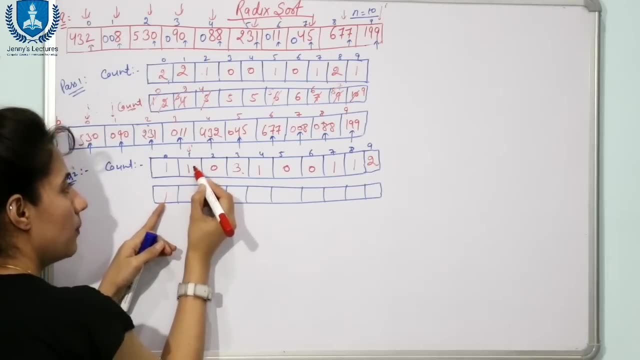 loop from 1: 1 to here k. k value is 9. here range is 0 to 9. fine, so how you will apply, how to find out that position, this 1 plus 1, that is 2. position would be 2, but index would be 1 in this array in. 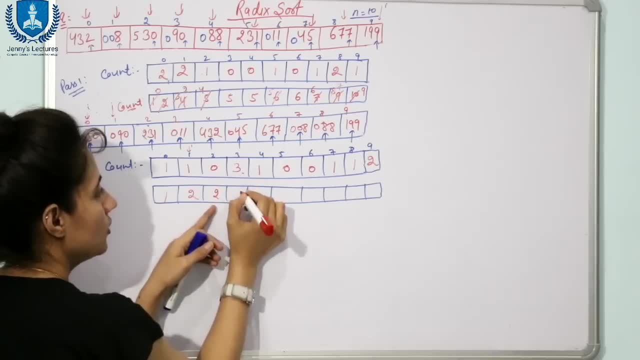 this array fine: 2 plus 0, 2, 2 plus 3, 5, 5 plus 1, 6, 6 plus 0, 6, 6 plus 0, 6, 6 plus 1 is 7, 7 plus 1 is. 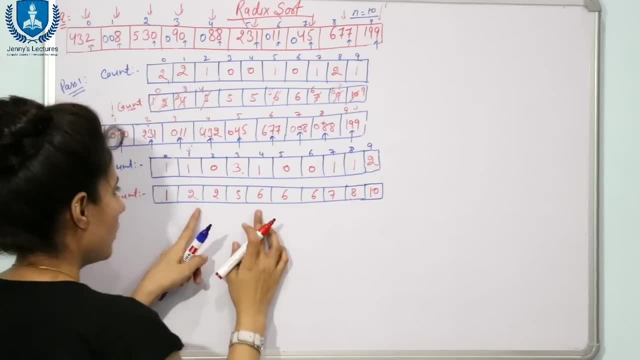 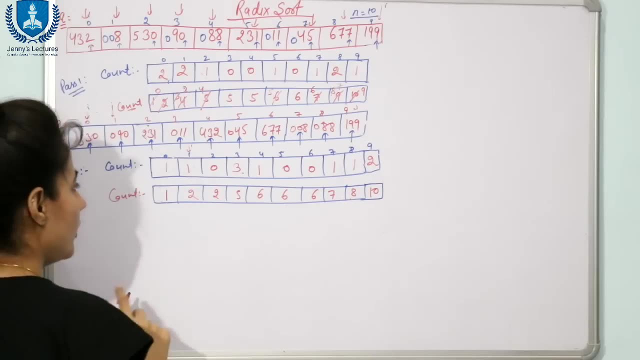 8. 8 plus 2 is 10, so this is now the updated count array. fine, now we are going to build. third step is: you are going to build the output array. you are going to take another array b. see, we have just this. we are going to update this array, this array. only it's not like that in the program. we are 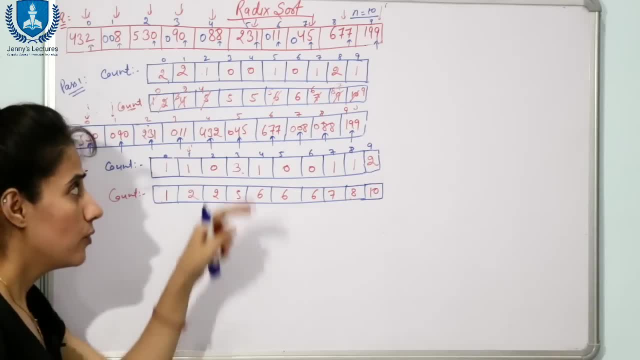 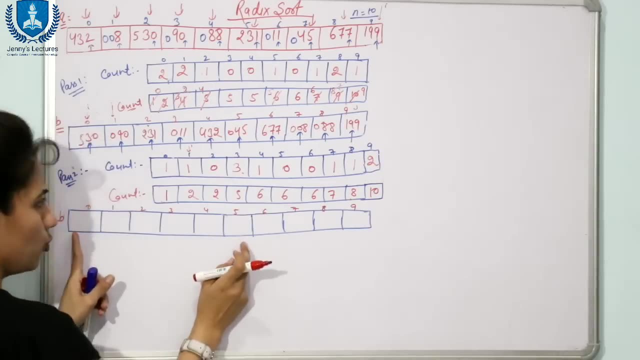 going to take one b array again, another b array. no, we have one b array only. we are going to update this array only. just i'm drawing the array again and again now how to build this output array. see, this is now our array. we are going to scan this. 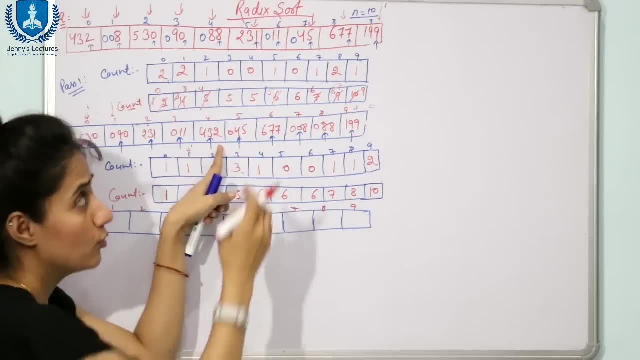 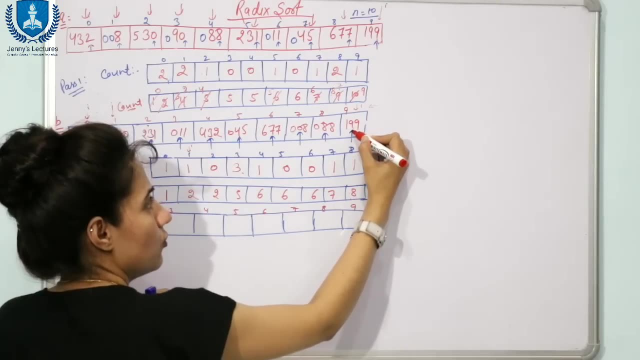 array from right to left: see the after pass one. this is the updated array. we are not going to check this array now. we are going to check this array. fine, now scan this one first of all. i is at this place now. we are applying count, so to this digit only we are going to check this array, this. 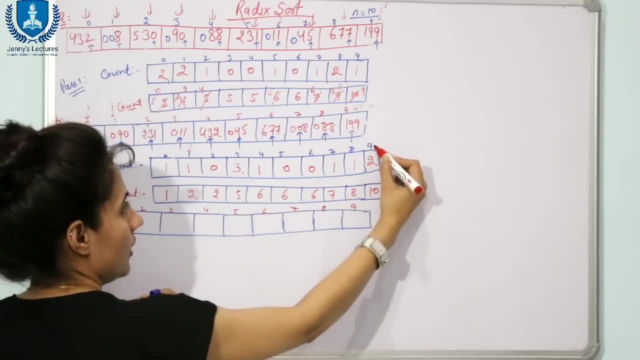 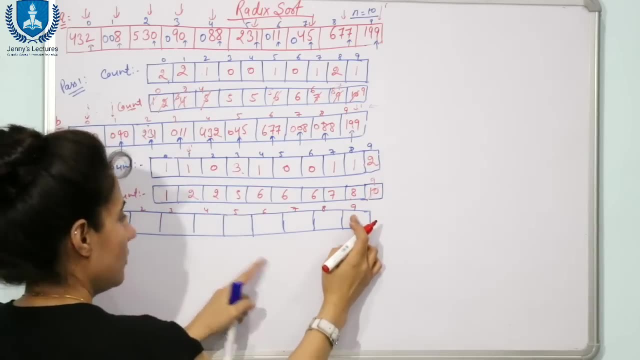 digit only. here we have 9, so go to the index 9, in count 10 and value is 10. but first of all we will decrease this, that is 9, and in this output array, at 9th index, we are going to store this: 199. see, this is the updated counter. you are not going to check. 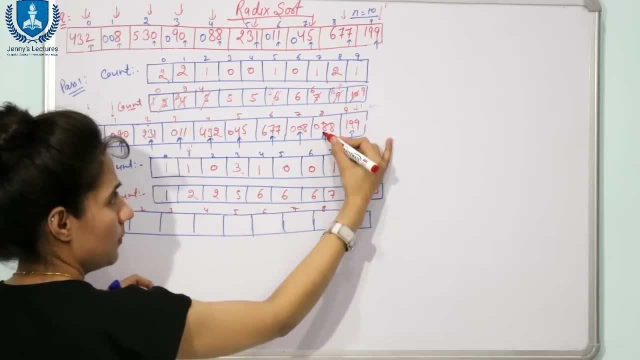 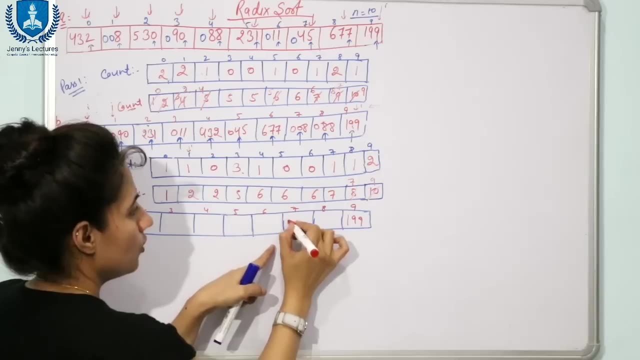 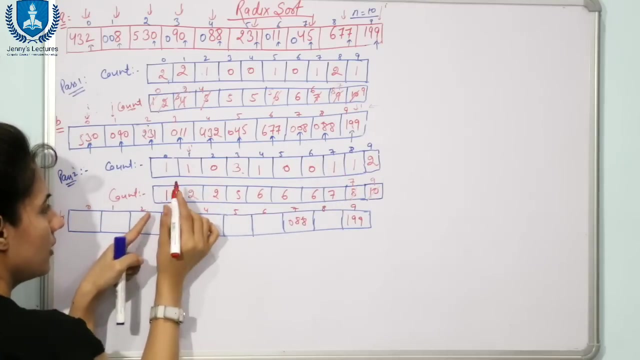 this one now, fine, decrement i here. second place digit is 8. go to the index 8. here we have value 8. decrement this, first of all, 7 at index 7. you are going to store 88 again. decrement this here at second digit. we have 0. go to the index 0. at here we have 8, and here we are going to store. 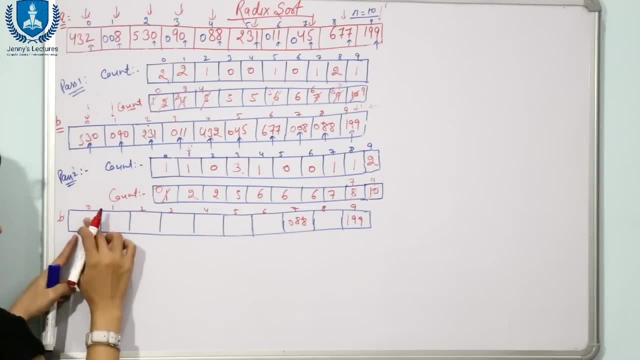 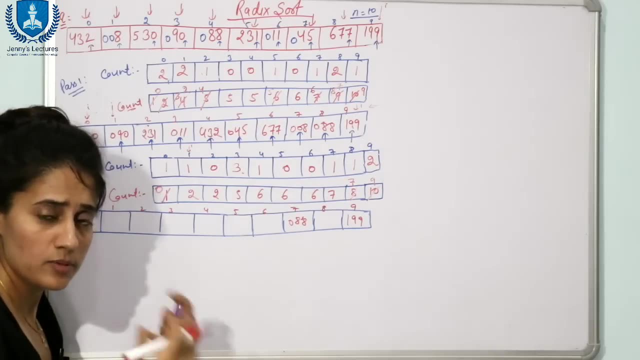 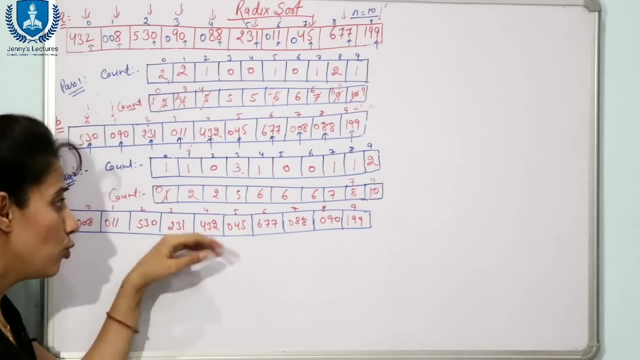 1. first of all, decrement this, that is 0, then go to the 0th index and store this value 8. fine, like this, same step would be applied and you are going to fill this array. so now, this is the array, output array. fine, we are just going to copy this. this, you know that numbers into the 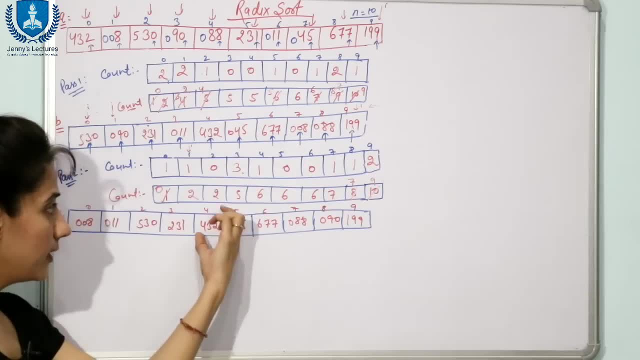 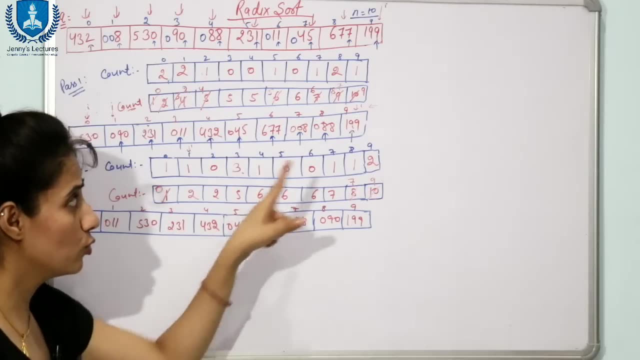 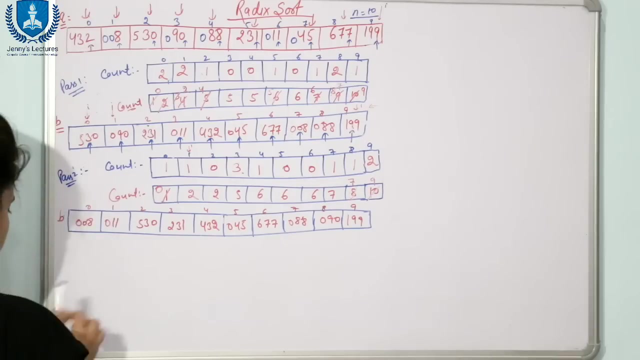 original array, that is a. so now, after pass to the updated array, is this, this one we have? just, we have applied counting, so two times, now one remaining. we are going to apply count sort on this digit, now this one on the digit which is at hundreds place. okay, now in pass 3, same steps would be applied. we are going to build this count array. 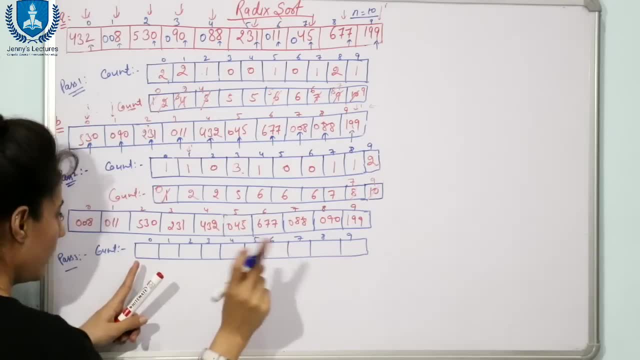 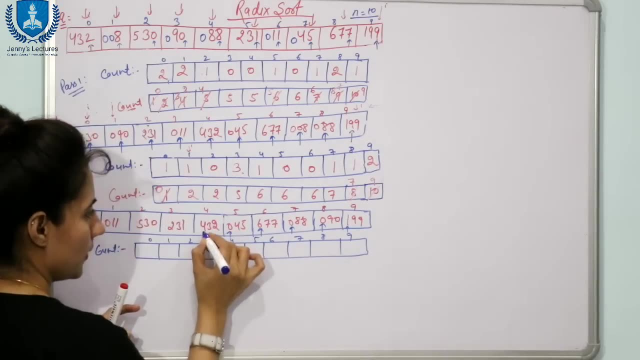 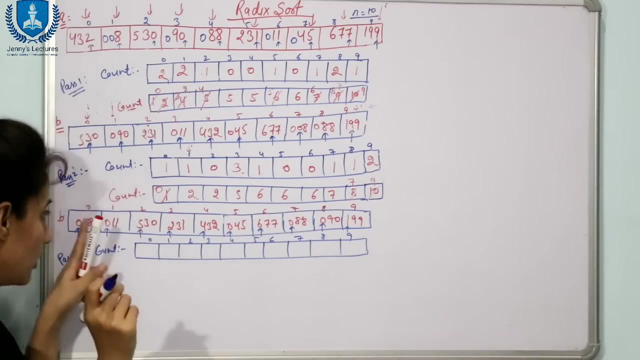 same size would be 10. we are. we are now applying the count sort on which digit, this one, this one, this one, that digit which is at hundreds place. so now count first of all. first step is we are going to count the number of times so you know, you can say frequency of this key value, this element. fine, 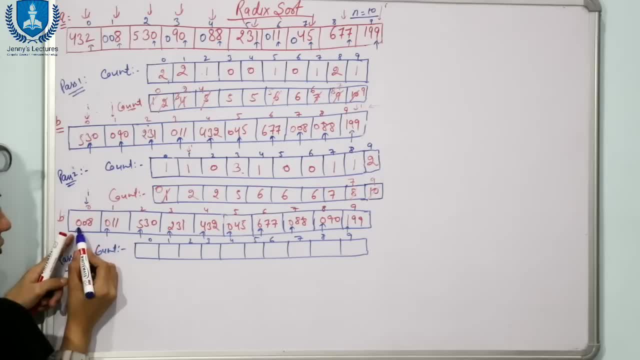 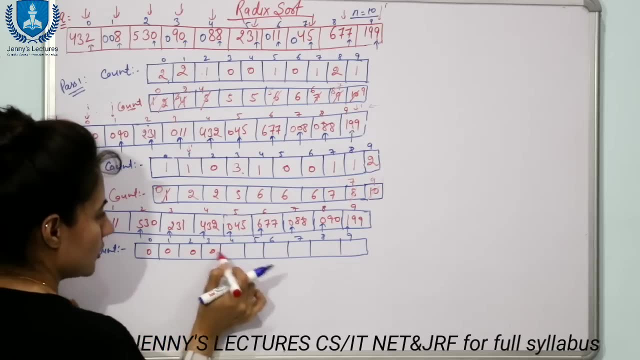 so now again, loop would be started from here. check out this digit. here we have 0, the value is 0. go to the index 0: see same steps. we are going to first of all initialize again this count array with 0. fine, now we are going to increment this value. 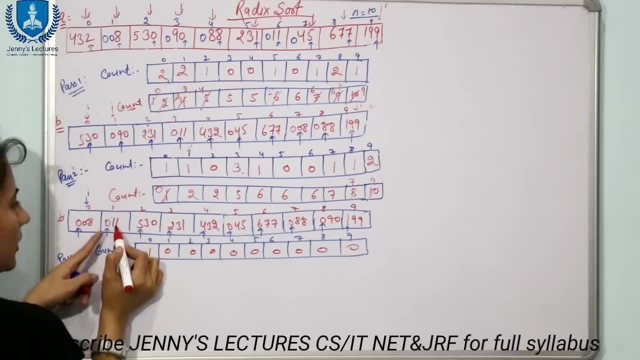 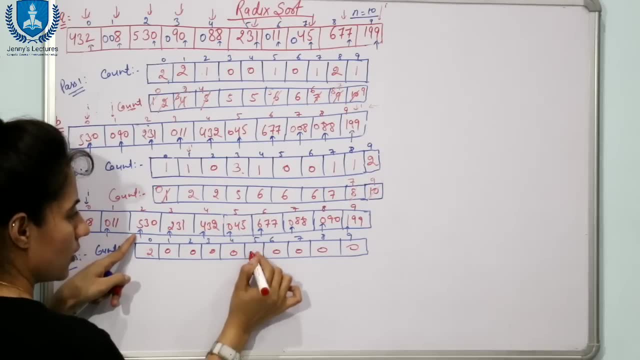 go to index 0. increment this value. now i would be incremented. here we have 0: go to 0th index: increment this value. here we have 5: go to index 5. increment this value. here we have 2: go to index 2. increment this value. 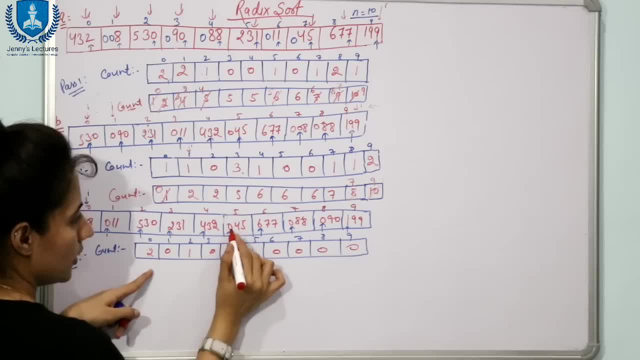 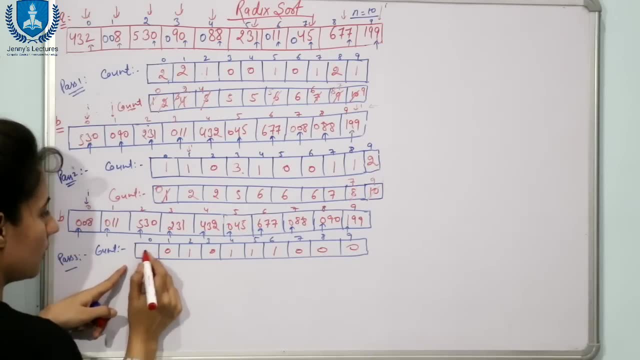 next, here we have 4: go to index 4. increment this value. here we have 0: go to index 0. increment this value. next is 6: increment this value 0. go to index 0. increment this value. next again: 0: go to index 0. 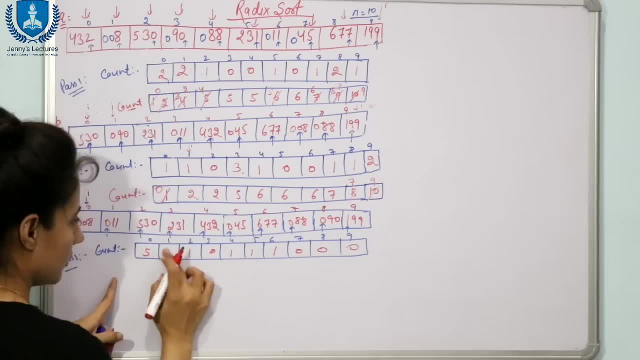 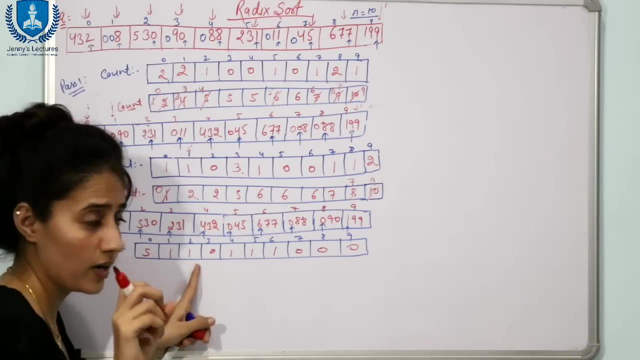 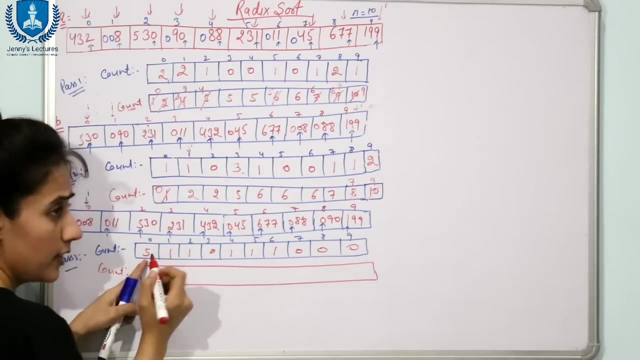 increment this value. and next is 1 index: 1- increment this value. fine, so this is now the count array. now we are going to update this count array just to reflect the actual position. so now the updated count array would be: see why we have 5 at 0th index. i guess you uh got the concept. see, we are. 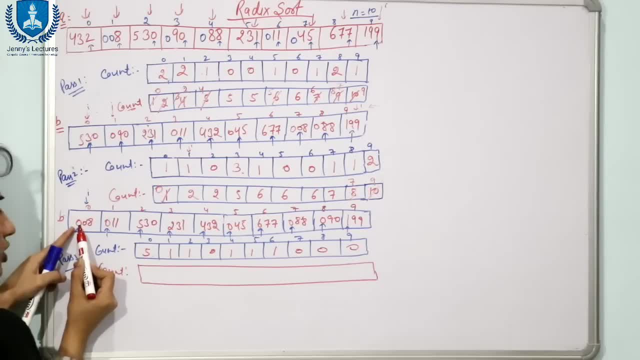 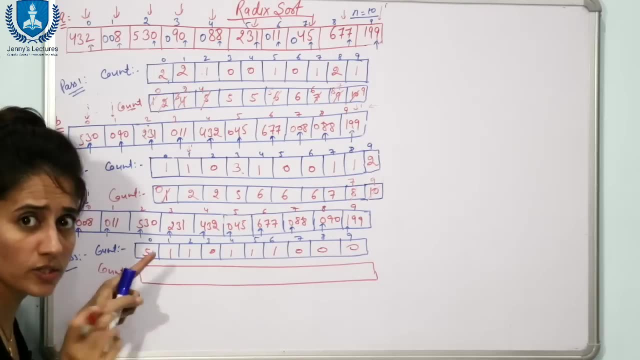 we are applying this count sort here only, so 0 at this place. how many times 0 is there? 1, 2, 3, 4 and 5 times. that is why the count today, the frequency, is 5 here. fine, so now we are going to update this. 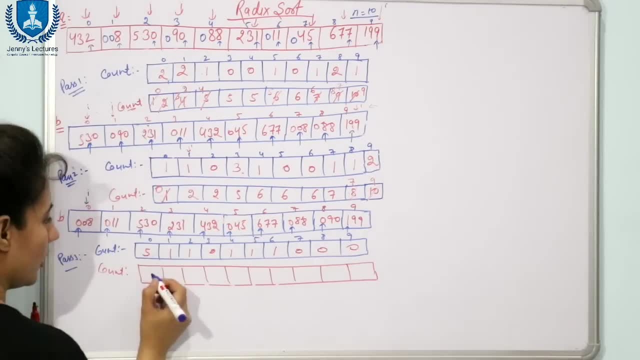 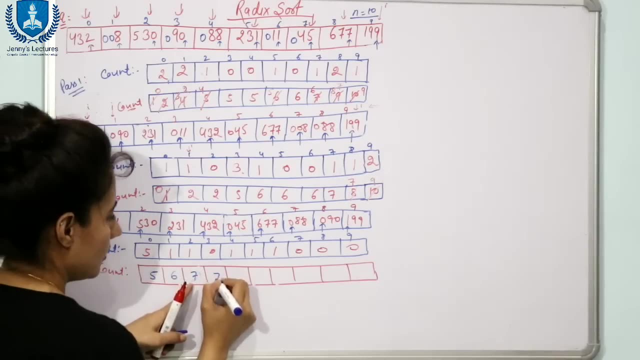 count array. how to update this first value would be, as it is 5, now 5 plus 1, that is 6, 6 plus 1, 7, 7, 7 plus 1, 8, 8 plus 1, 9, 9 plus 1, 10, and here we have 10, 10 and 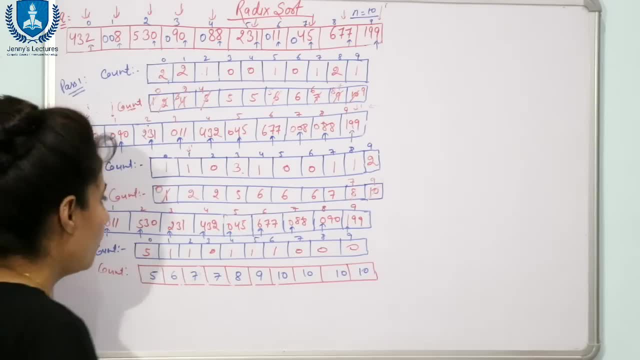 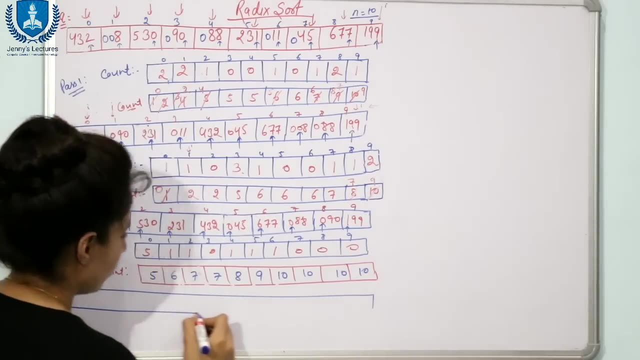 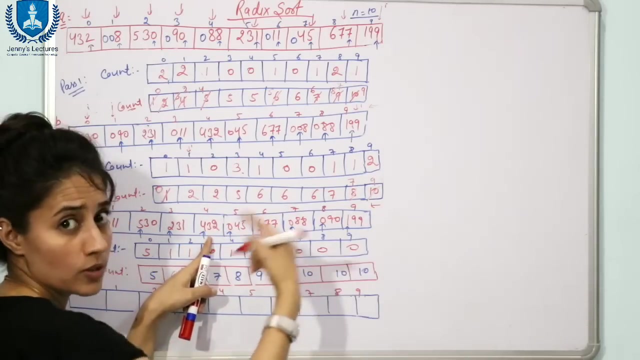 10. now this is our updated count array. now we are going to build the output array same. another array is there, that is b array. you are going to update this b array. only see: now this is the operated array of after pass 2. so we are going to scan this from this right to left. so 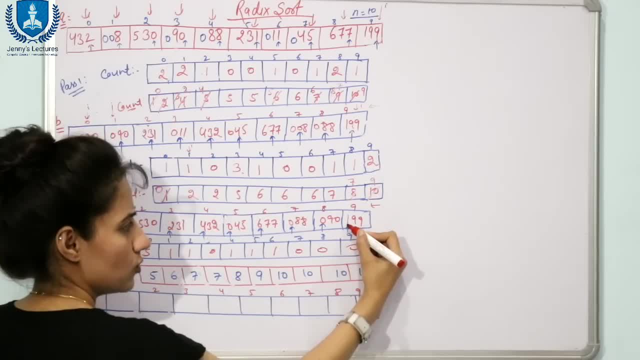 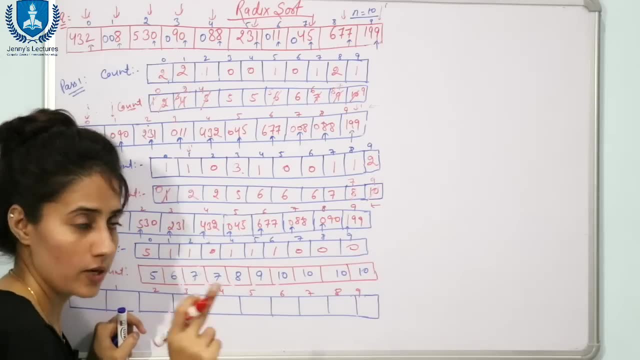 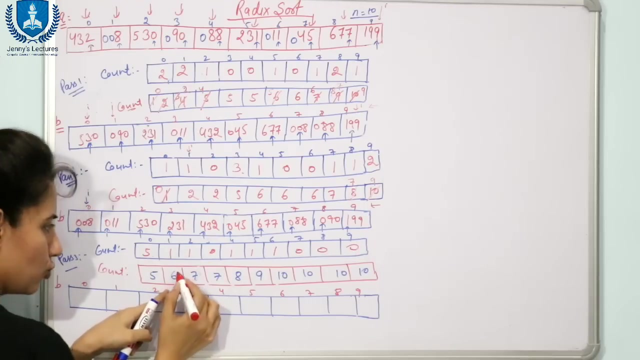 start from here, the value at index this, this the hundreds place, because in this pass we are applying this counting sort at this digit only. so here value is 1, go to index 1 and the value is in: count sort is 6. so we are first of all decrease this, that is 5. at 5th index we are going to store: 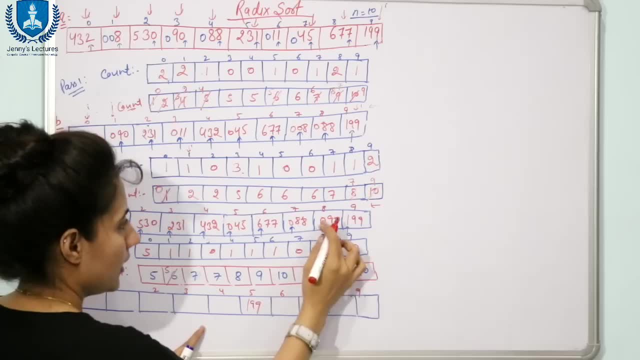 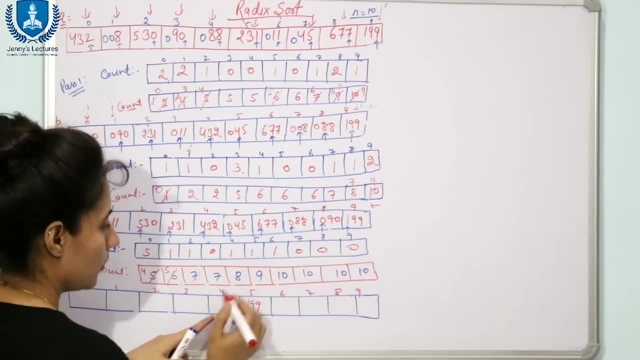 199. fine, now again decrement this: i. here we have 0. go to the index: 0. here we have 5. decrement this, that is, 4 at 4. we are going to place 90. now decrement i: value: here we have again 0. go to. 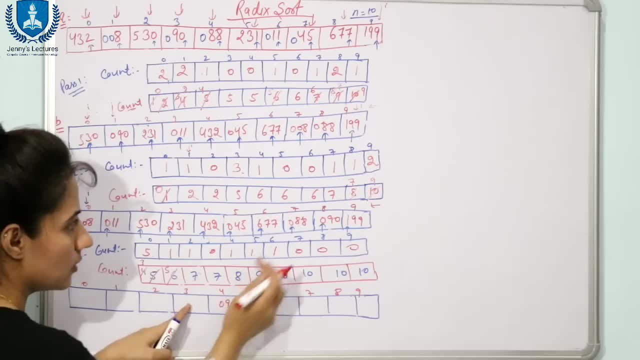 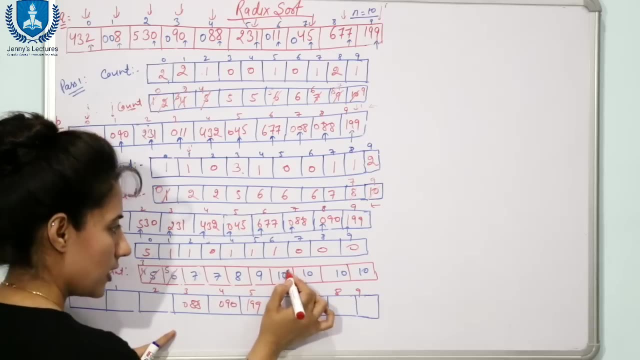 index 0 in decrement this: that is 3. at 3rd, we are going to store 88. now decrement this: here we have 6. go to index 6. value is 10 decrement this: that is 9. at 9th index, we are going to store 677. 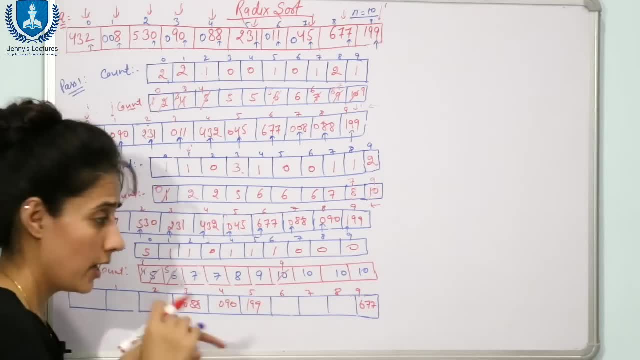 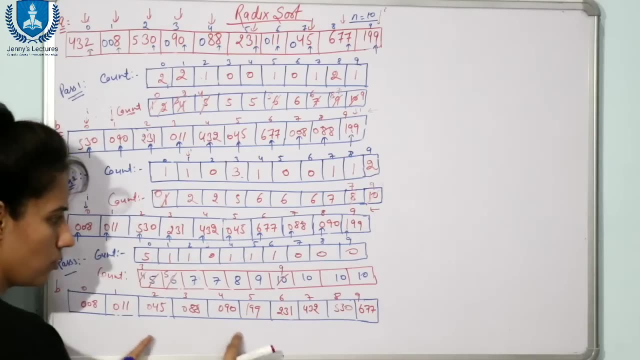 like this: we are going to follow the steps and now, finally, you get the sorted array. so now this is our output array after pass 3. as you can see, this array is now sorted. you simply copy the element of this, this array, the b array, into array and you can see that this array is now sorted. so now this is our output array after. 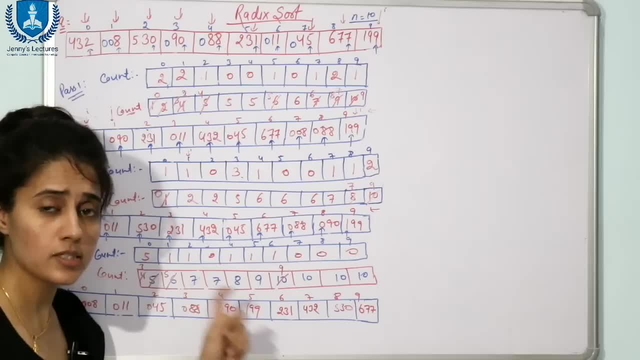 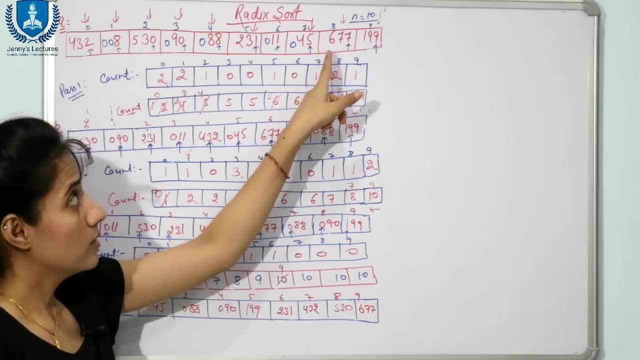 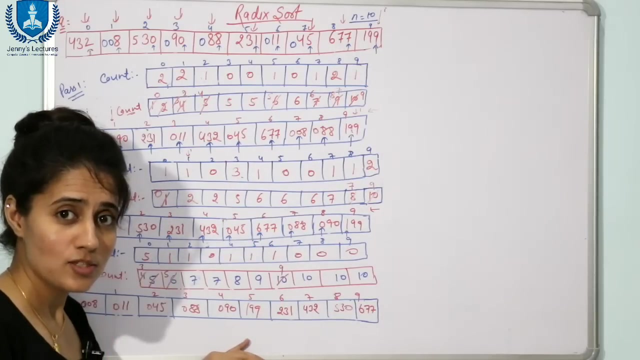 a, the original array and you got the sorted array. this is how we are going to apply the radix sort. see how many times you applied counting sort here three times. why three times? because in the maximum element in the array the number of digits are only three. see, i tried my level best. 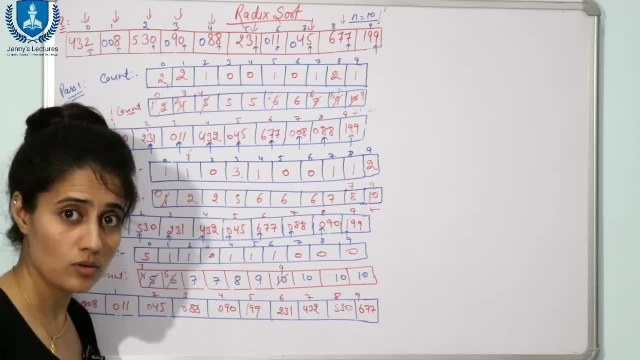 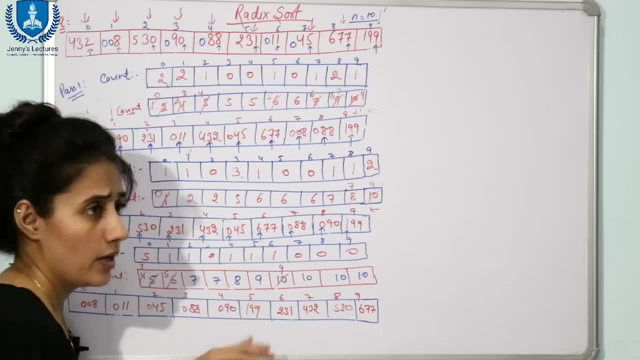 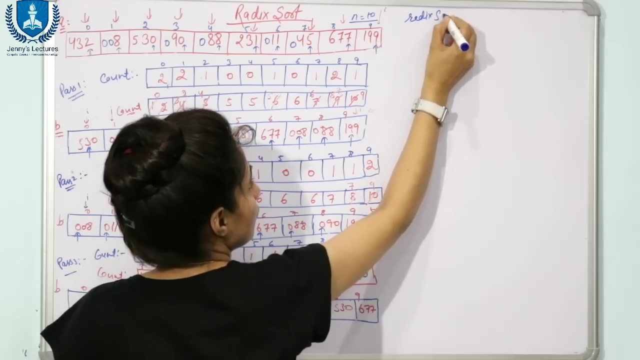 to explain this radix sort in a easy way. i hope you got the concept. if you got the concept, then please let me know in the comment box. fine, see now. now we are going to write down the code for this radix sort. so we will take one function that is radix sort. in this you are going to pass array a and 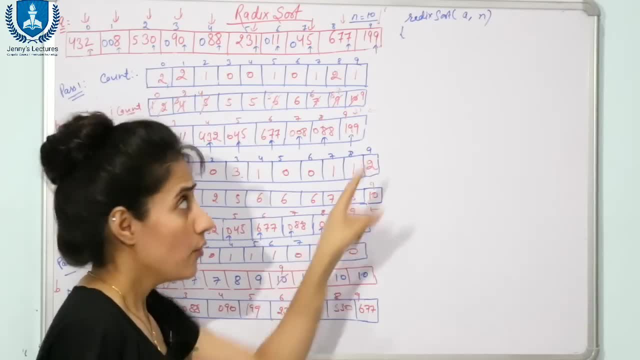 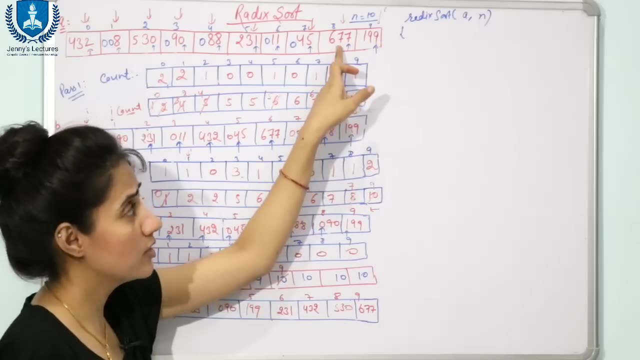 number of elements in that array. so now in this radix sort we are going to call what counting sort and how many times. for this example, three times, because maximum element is this one and the number of digits in this element is three only. maybe in another case you have, maximum element is 1432. 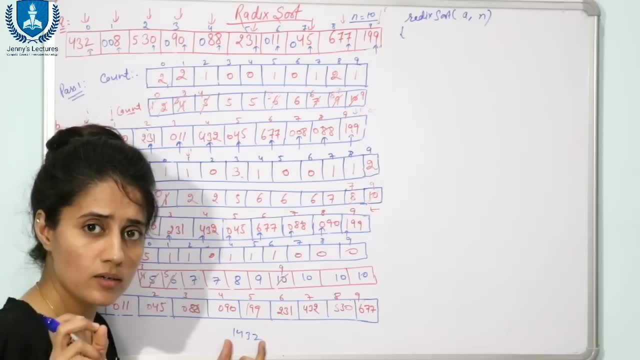 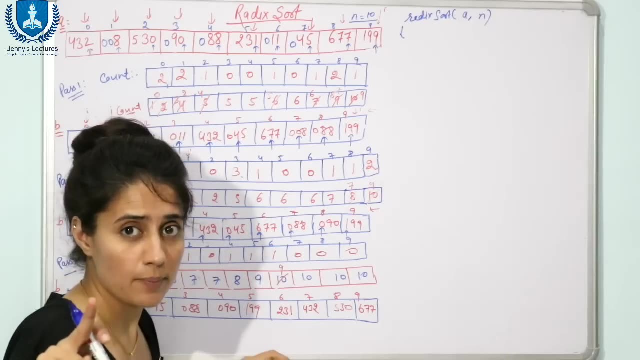 so here, in maximum data, the number of digits are only three. so in this case you are going to call four. so four times you are going to call the count sort. so first of all you are going to find out the maximum element, right? so you are going to write down a function i am not going to write down. 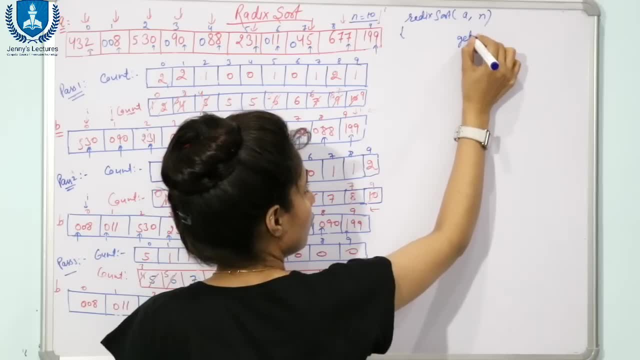 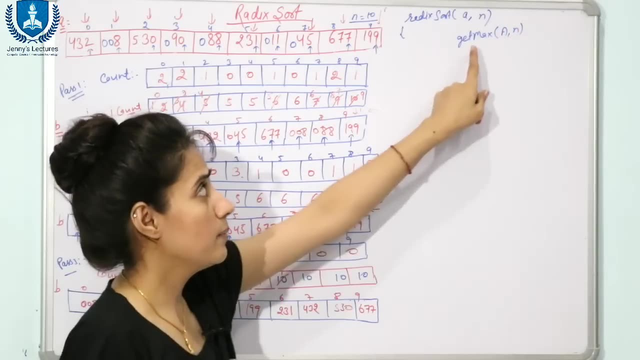 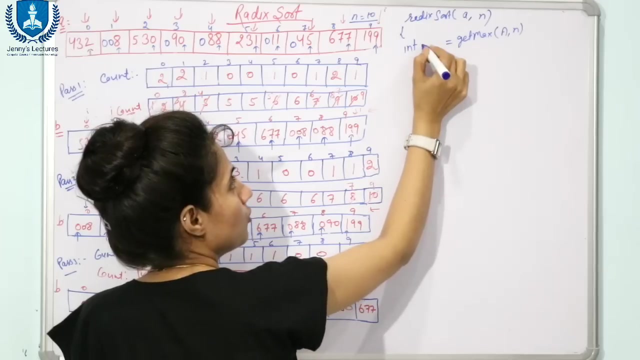 the code for that function. i am simply write down that function. suppose we are going to take get mix a function. we are going to pass array a and number of elements and this get mix will return the maximum element, this array. so we are going to store this into a variable. suppose mix: 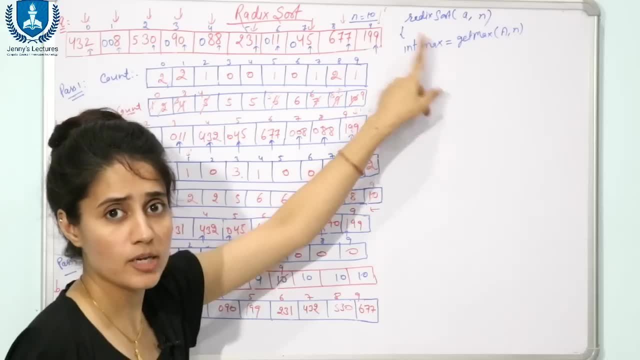 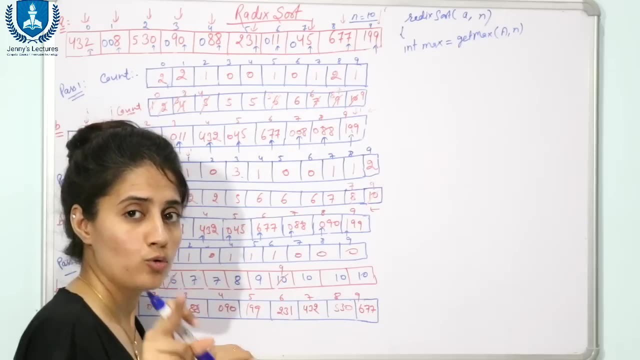 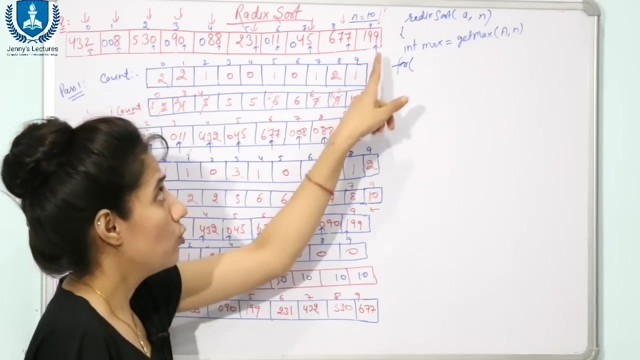 fine, in max, now we have the maximum element. so in this case, max in max, we have the 677. so now you are going to apply a for loop. fine, see, we are going to call the counting sort on the position, first on this position, then this position, then this position. once tens and hundreds. so i am going 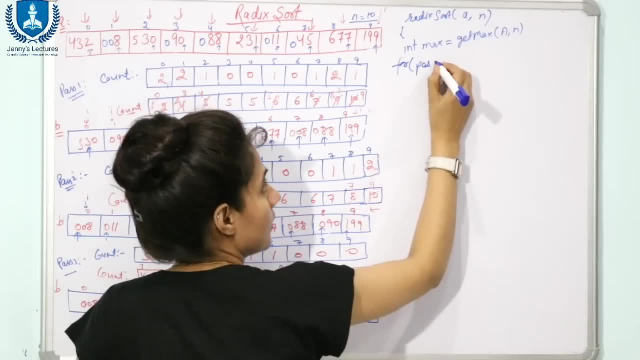 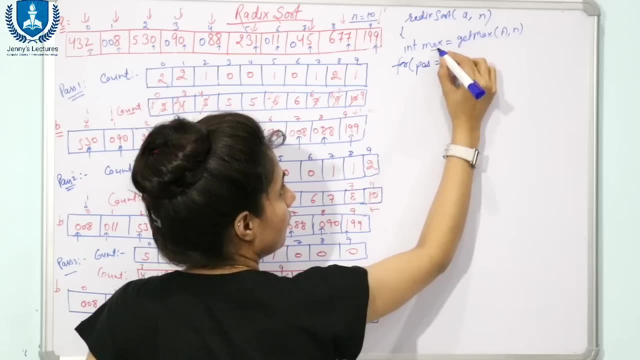 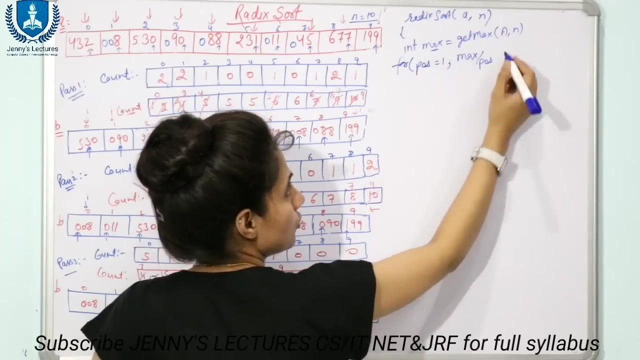 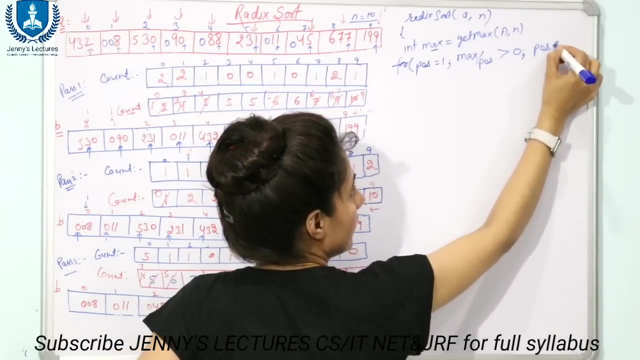 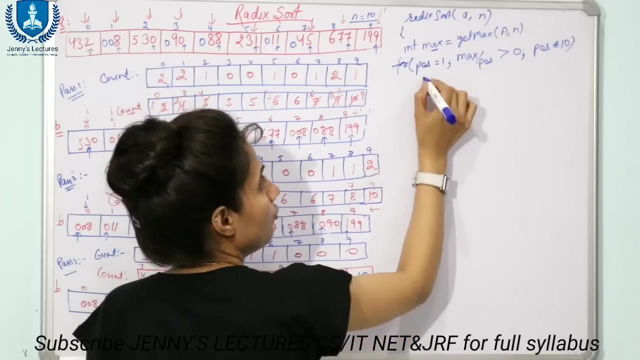 to take a variable position, or you can say pos. i am going to initialize it with one. and now the condition is here: we have the maximum data in variable max max divide. by this this pose is greater than 0 and this pose would be incremented by into 10, not plus 10 into 10. and now we are going to call this: 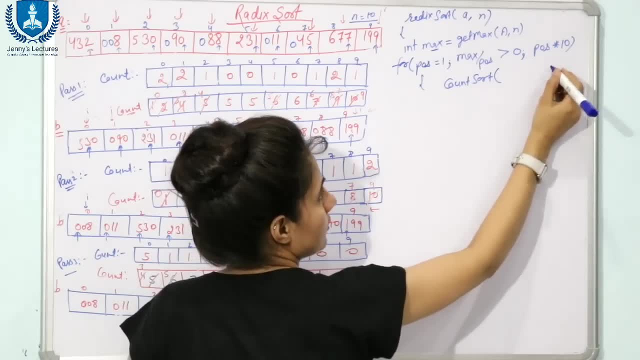 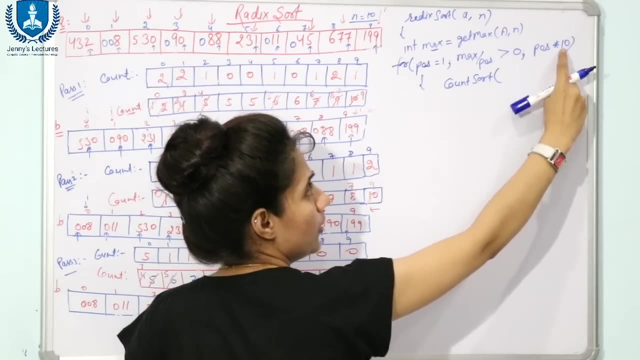 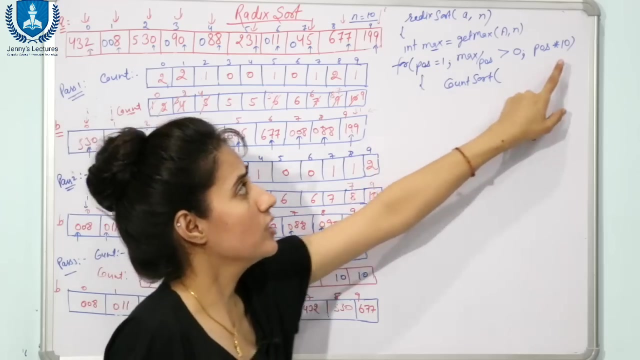 count sort. so we are going to pass some arguments here. i am going to tell you that thing later. first of all, why you are incrementing. incremented this post value into 10. see first of all position: is this one position? next position is tens, so one. the next position is 10. next position is hundreds, so 10 into 10, that is 100. that is. 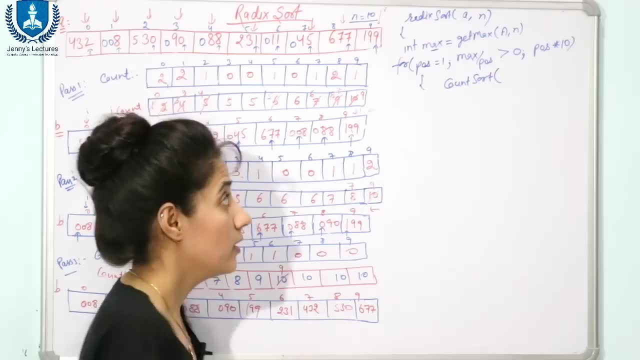 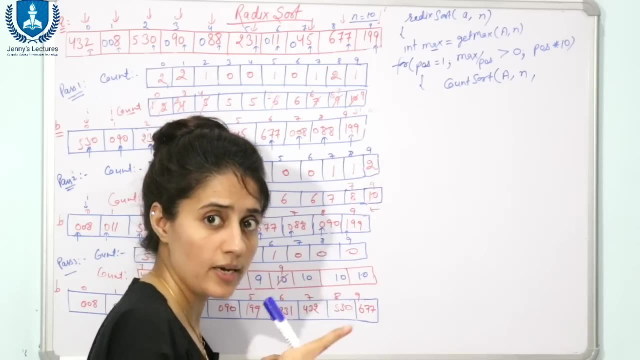 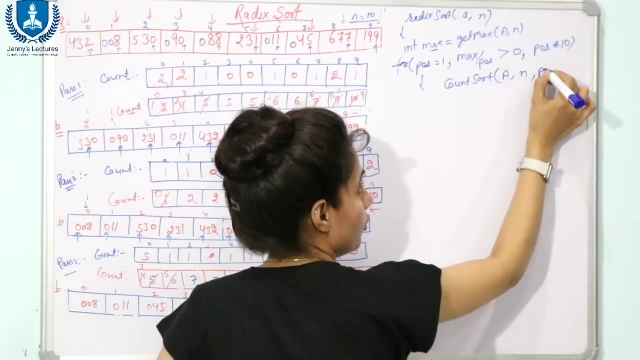 why i am incrementing this into 10. fine, now in count sort. in count sort you will pass array, a number of elements in the array, plus this, this value, this position, value at which position you are supposed to call this count sort. so you are going to call at pos position first of all, once, then tens, then 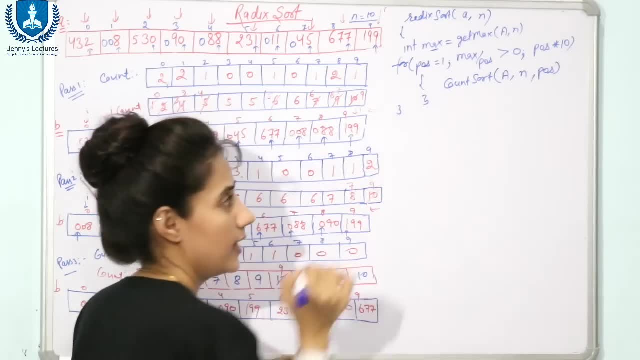 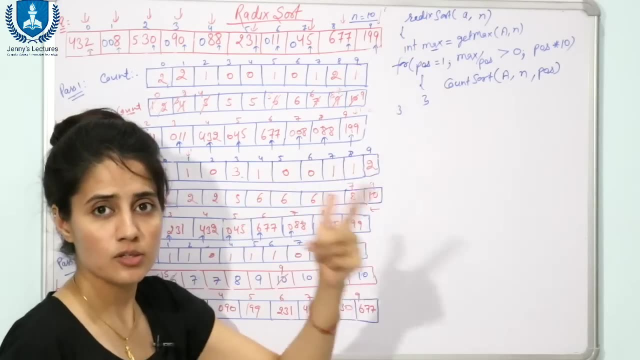 hundreds would be passed. and this is it. so this is the code for red x sort. now we are going to write down the code for this count sort in main function. you are going to call this red x sort. see, in this case, if you call this red x sort, then in this, out of this array, the 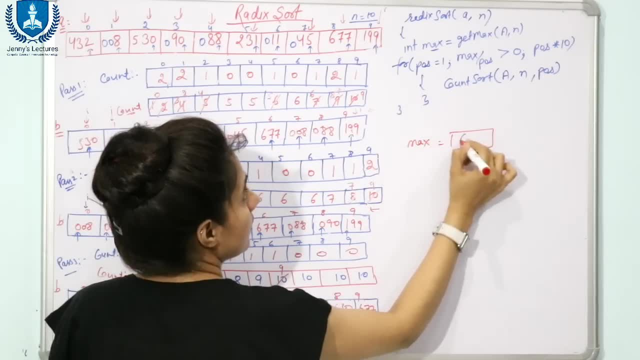 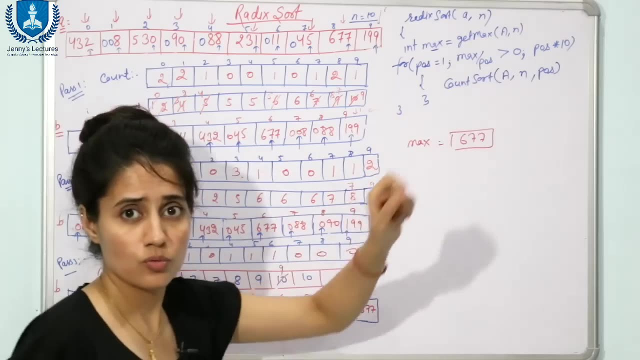 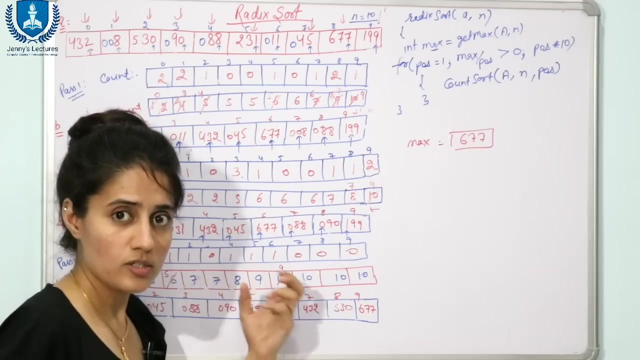 maximum. the value of this maximum would be 677. get max would be a function. you are going to write down the code for this function also to find out the maximum element out of this array. i guess you can write down the code, because here the main, you know, logic is about this red x, or so i'm not going 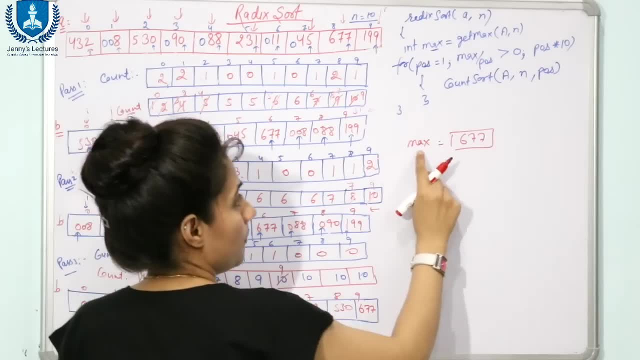 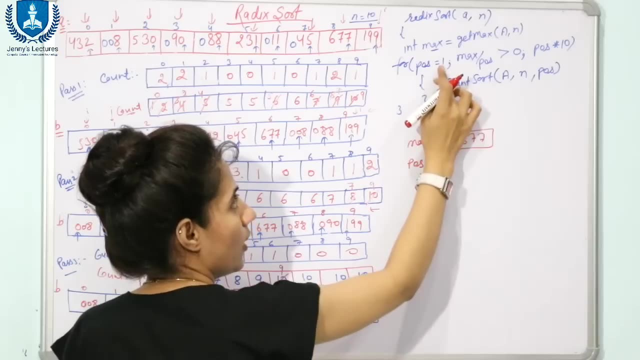 to write down the code for this: get max. fine, so maximum is 677. now in for loop. see, we are going to take one variable and the value is one. see, we are going to take one variable and the value is one. see here, max divided by post max is 677 divided by 1, that is 677. only that is greater than. 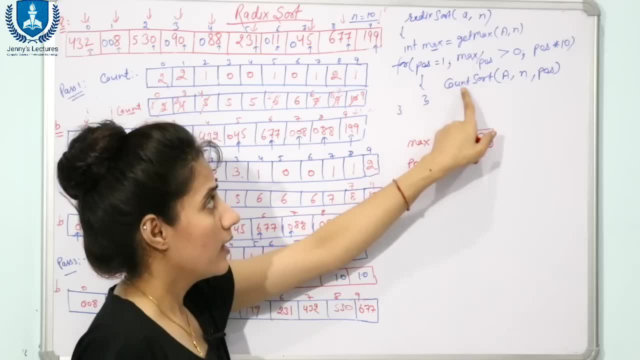 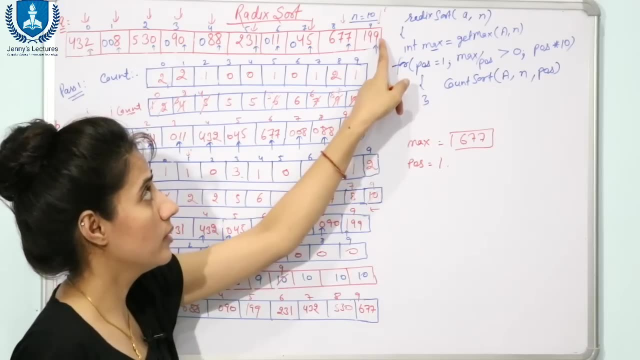 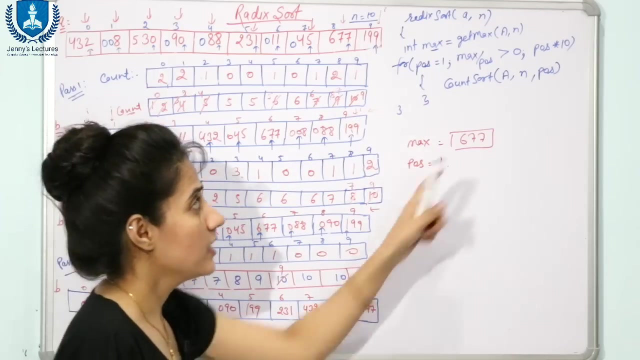 0,, so value is condition is satisfied. call this count sort. array would be passed n and post value is 1, so 1 would be passed. so now counting sort would be called in this, from this position, at this position. fine, now next. next this after: after the completion: 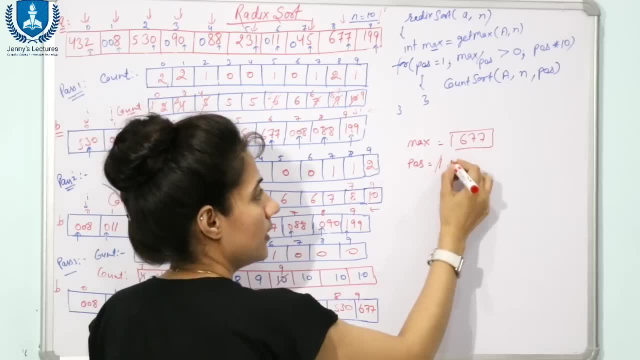 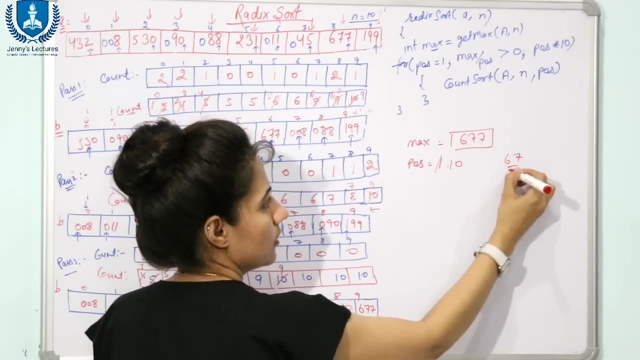 of count sort. this post value would be incremented. now, post is what? 10, now max divided by post. max is 677 divided by 10, that is 67. only fine, 67 is greater than 0,. again, count sort. 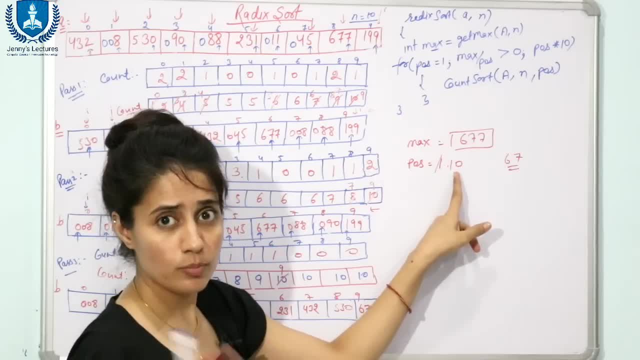 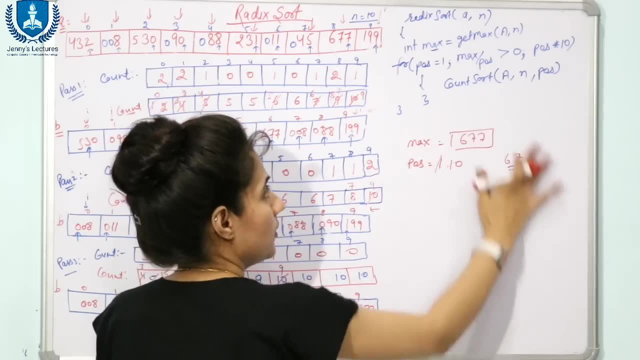 would be, post would be called and post value is 10, 10 would be passed. so at this place this count sort would be called now. next is after the completion of count sort. now, post value is 10 into 10, that is 100. 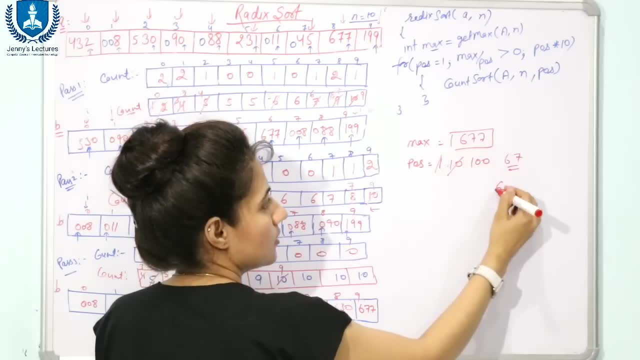 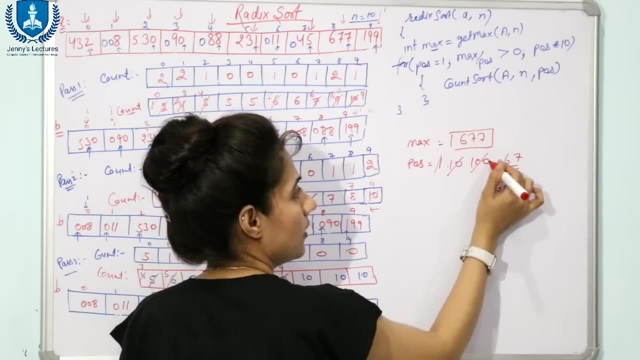 677 divided by 100, that is 6. only 6 is greater than 0, now again count sort would be called now after count sort. again, post value would be 100 into 10, that is 1000, now 677 divided. 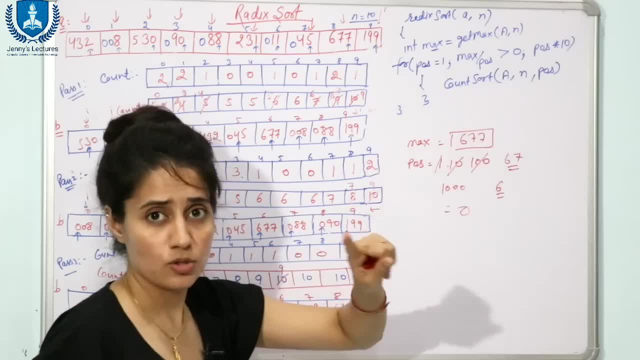 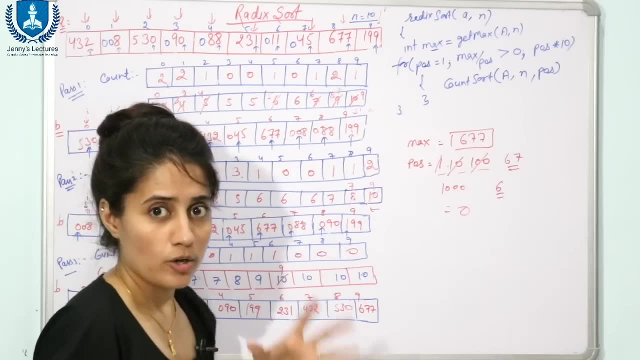 by 1000, it is 0, now 0 is not greater than 0, now count sort would not be called. now how many times this sorting would be called: 1,, 2 and 3 times. so I hope you got the working. 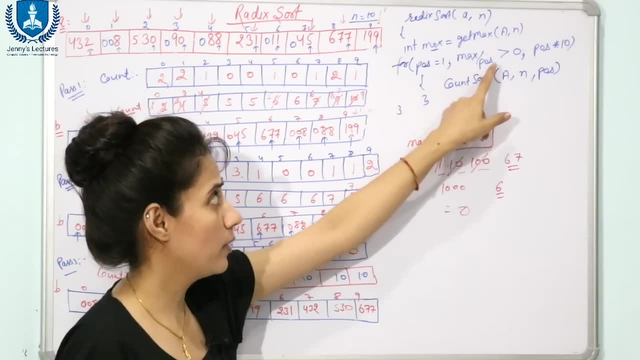 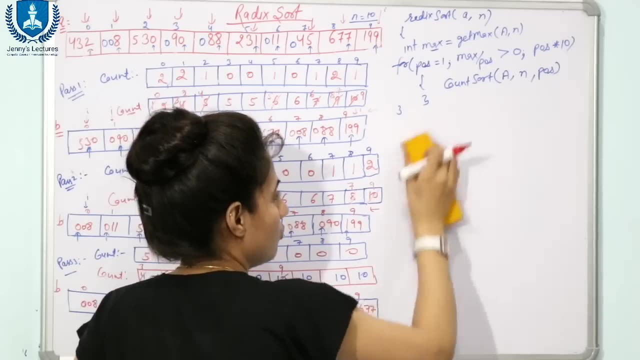 of this for loop, Why we have written this max divided by post greater than 0,. now we are going to write down the code for this count sort. we have discussed the count sort 4, 4 loops would be there. you have just do. 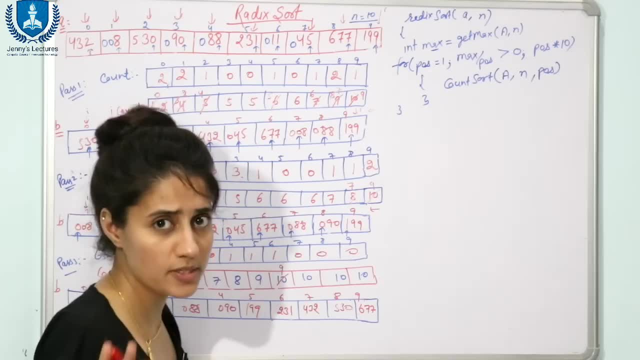 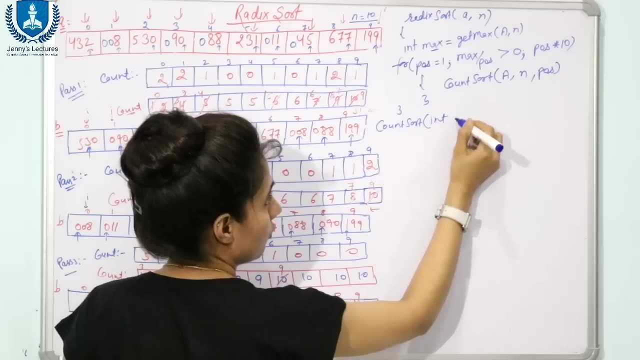 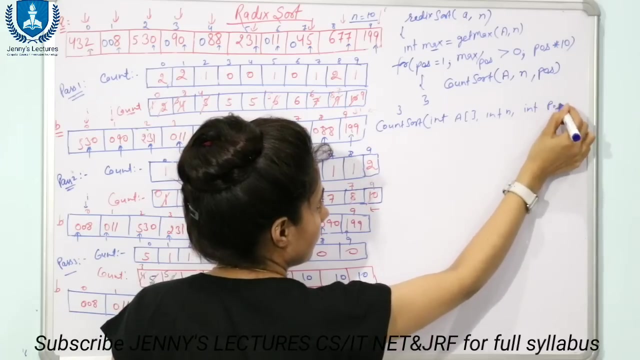 a little bit modification for this radix sort, logic would be same. fine, now we are going to define this count sort. so here you are going to take what int of this array, a int, n, you can say, and int. Now write down the count sort 4, 4 loops would be there. now start with the first. 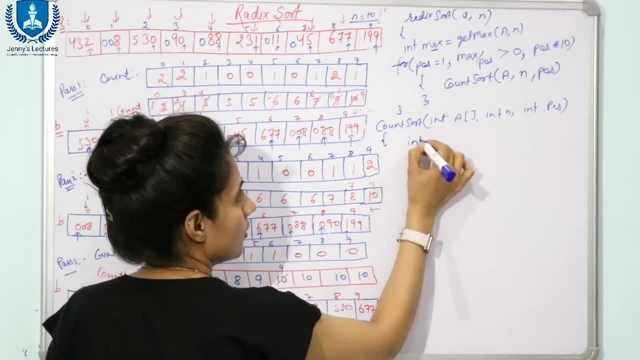 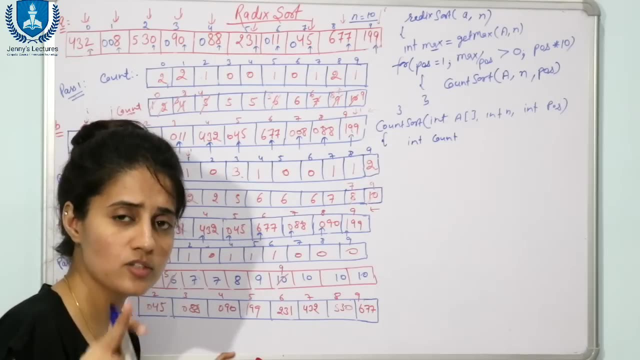 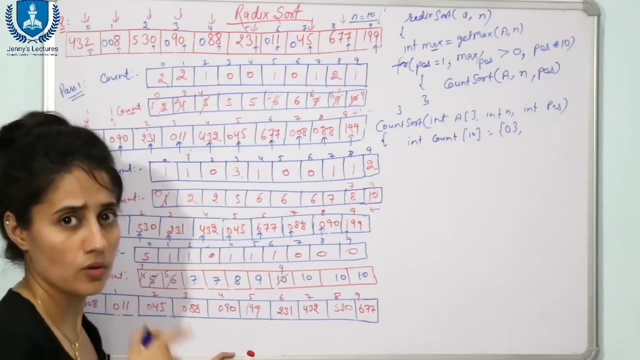 step is just take a count. you can say this count array and the size of count array is here- is fixed. that is 0 to 9 range. so count array would be 10, so just take 10, size is 10 and initialize it with 0 first of all. that is the first step in this count sort. 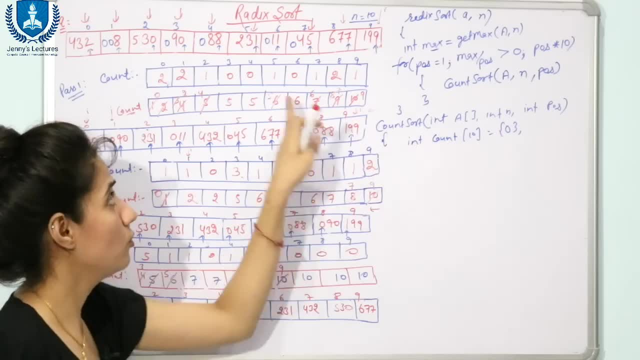 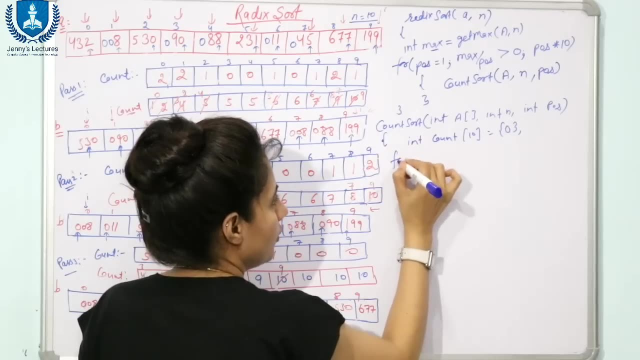 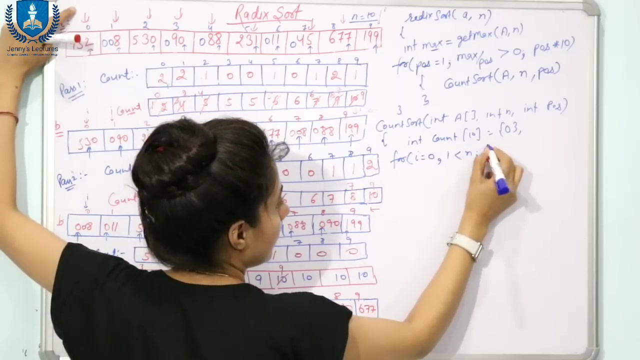 function. Next step is now you have to fill this count sort array. How we are going to fill. We are going to count the frequency of the elements. now one 4 loop would be applied. we have started. i is equal to from 0,. i would be less than n and i++. so now what we have. 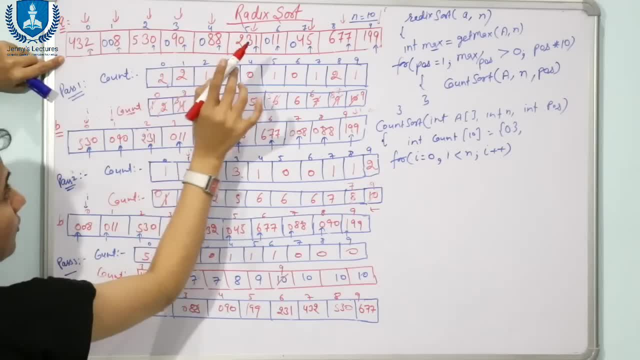 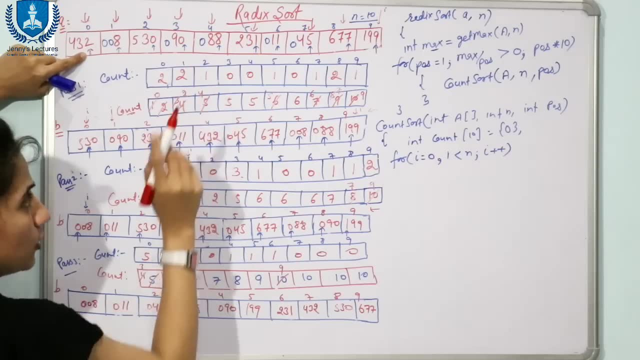 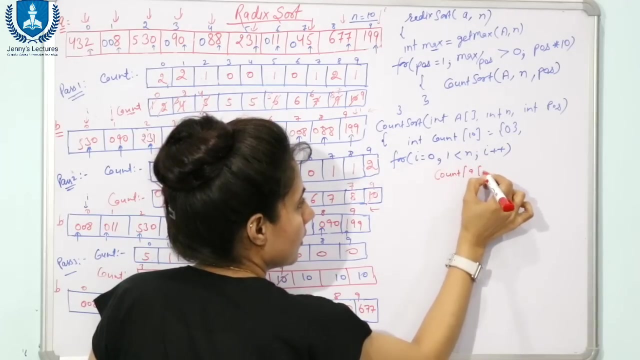 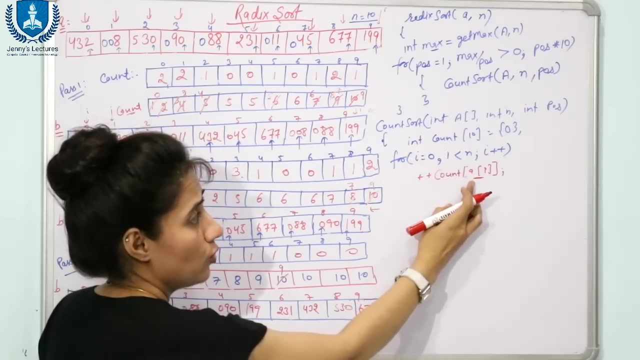 done here. see, in first pass. in first pass we have just taken this value, that is, 2, we went to the index 2 and increment this value, simply fine. So in count sort what we have done, We have written count a of i and you can say plus, plus. see, this logic would not work. 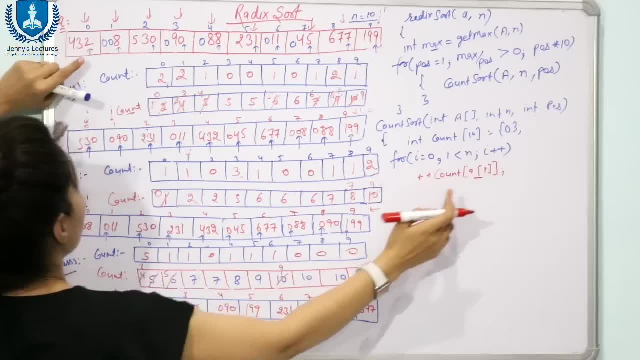 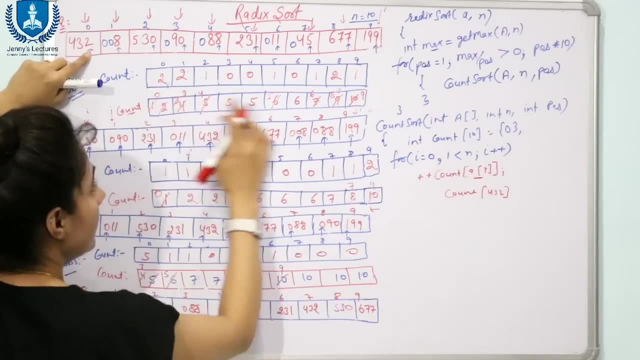 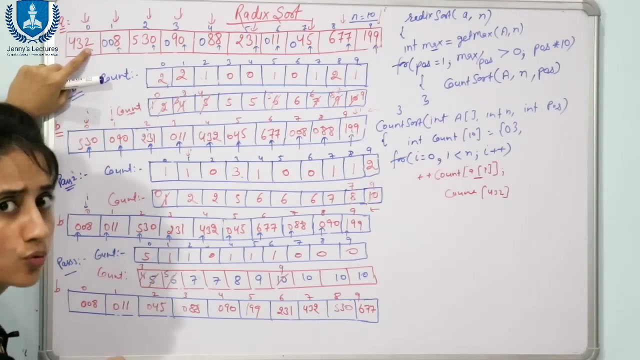 here. why? So, because see, a of i i value is this one: a of i is 432, so count 432, but we don't have any index 432, so we are, we are just, we have to just take this value, this 2, we. 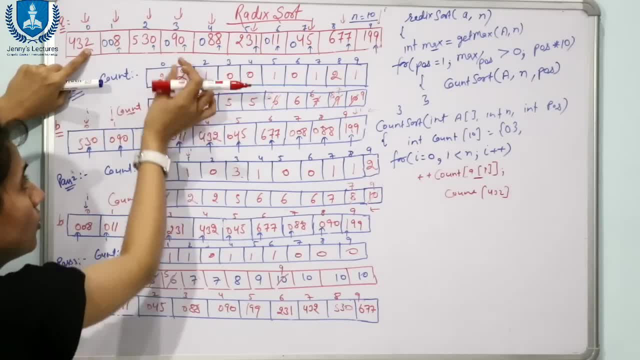 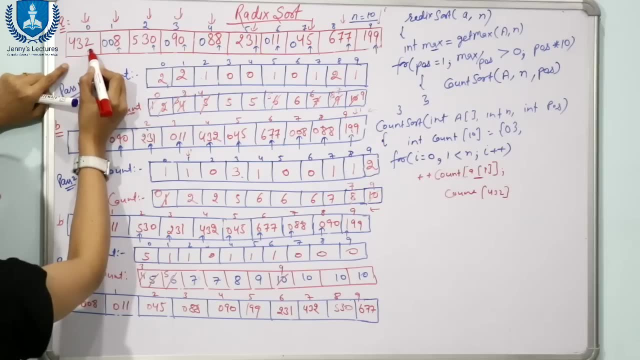 are concerned with this. So we are concerned with this value, only this one, this one, this one. we are not concerned with the complete value. all the 3 digits? no. So you have to, you have to find out this digit from this number. now, how to find out? 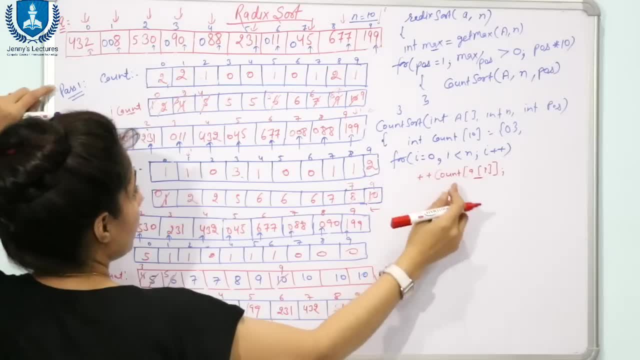 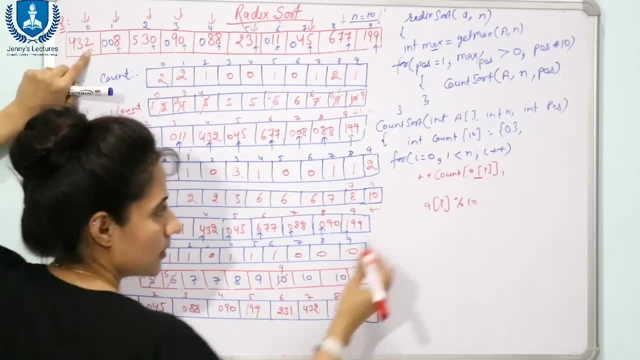 this digit, what is the logic, So what you can say, to find out this digit, out of this number, you can say: we just do a of i mod 10 and here we can write count. So a of i is 432, 432 mod 10.. 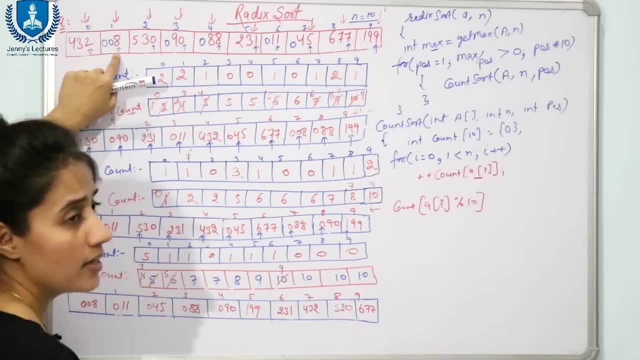 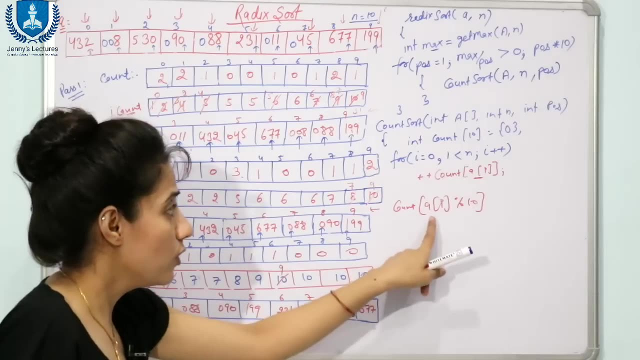 That is 2, a of i is 8, 8 mod 10 is 8 only this mod 10 is 0 only. so that is fine, but this will work only for pass 1, because see in second pass, in second pass you are going. 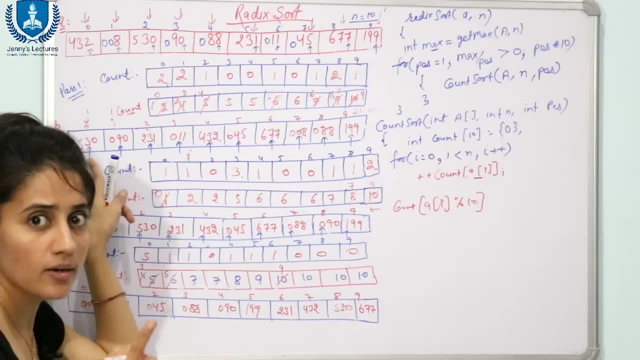 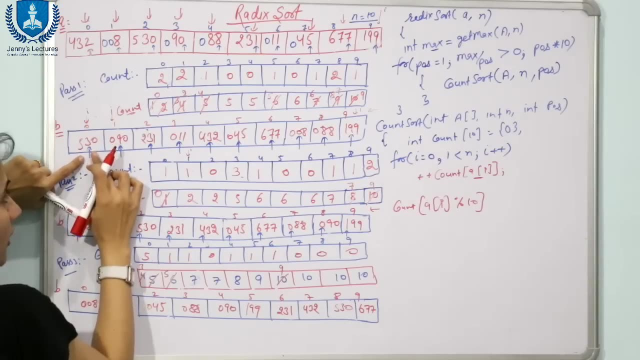 to deal with this digit, the digit which is at 10th place, but according to this logic, in second pass only when i would be at this place when you are going to start here. then 530, 530 mod 10,, that is 0.. 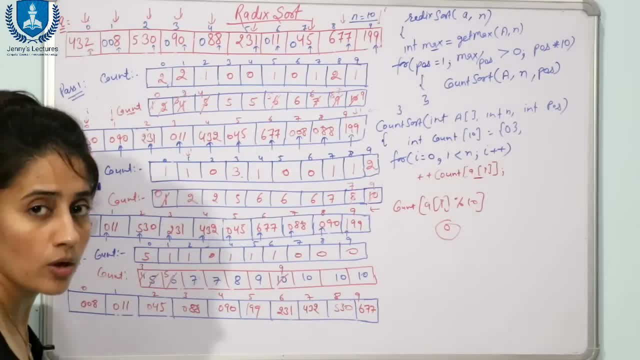 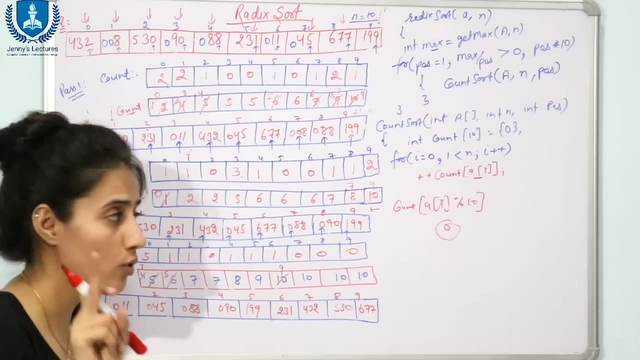 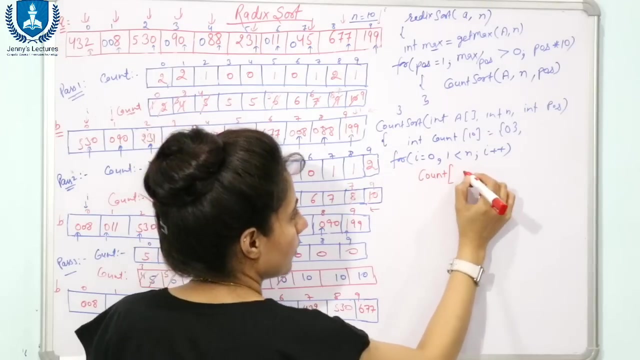 But we are going to take 3, now we have to take 3, so now what you will do. so this thing is somewhat right but not exact. you have to modify this thing also. now what you have to do. see, you will have to write within this for loop. so now this is the exact logic. 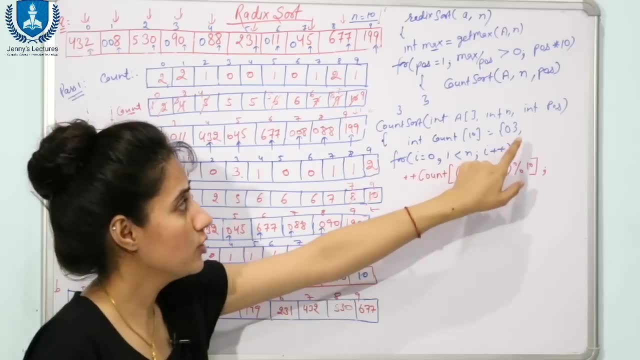 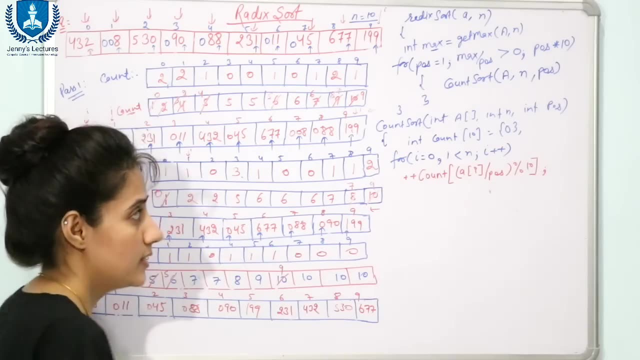 you have to divide this number a of i by this value, this position value. then you can do this. after that you can write this mod 10.. See, in first pass it will. in second pass, I am going to check. see, the value is 530,. 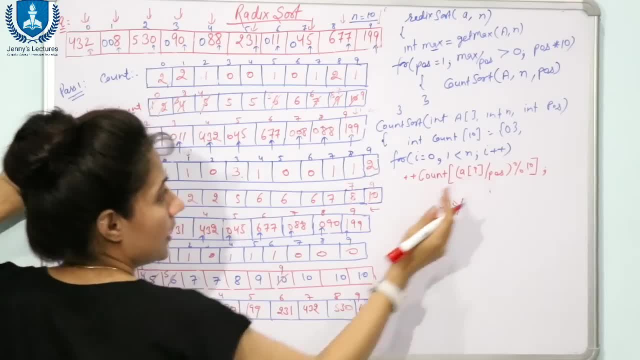 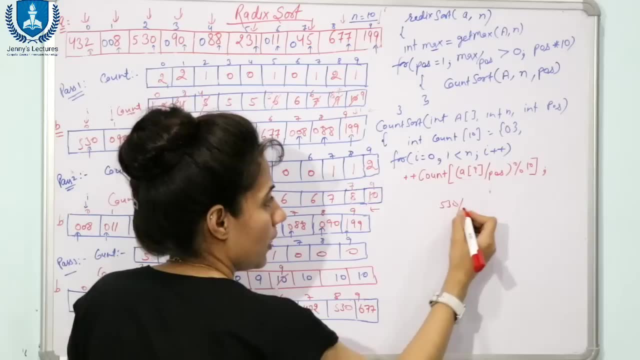 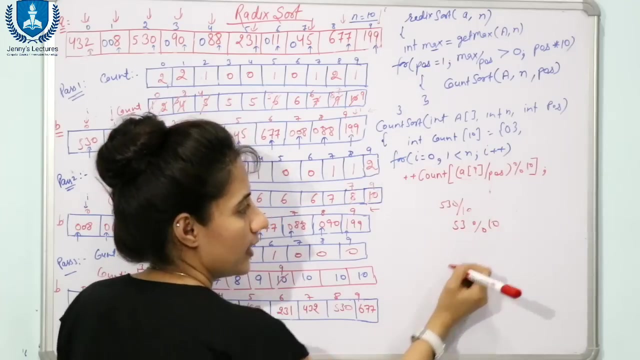 530, a of i is 530 divided by in second pass. in second pass, this pos value would be would be incremented and it would become 10.. So 530 divided by 10, it means it becomes 53 and 53,, 53 mod 10, so it becomes 3 and. 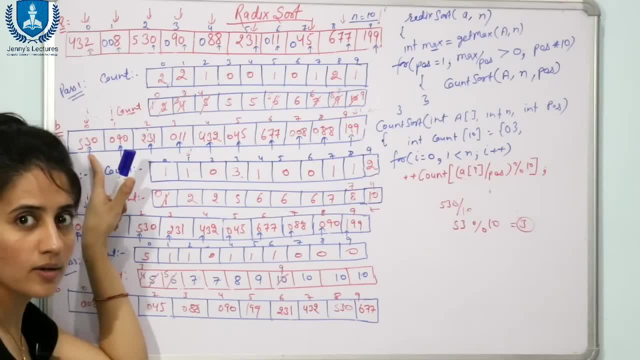 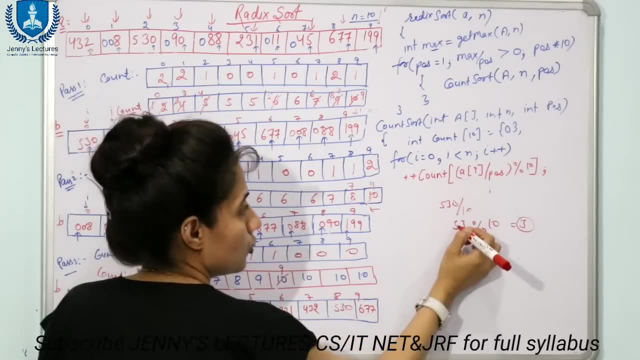 obviously it is 100.. and obviously we want this 3 only. fine, in third pass you can check. in third pass the post value would be 10 into 10, that is 100. so in third pass you can check again. suppose we are going to take. 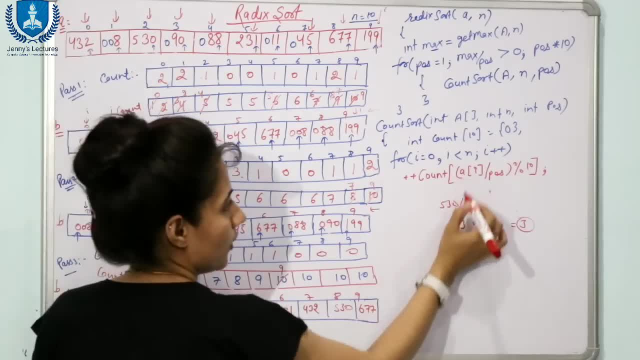 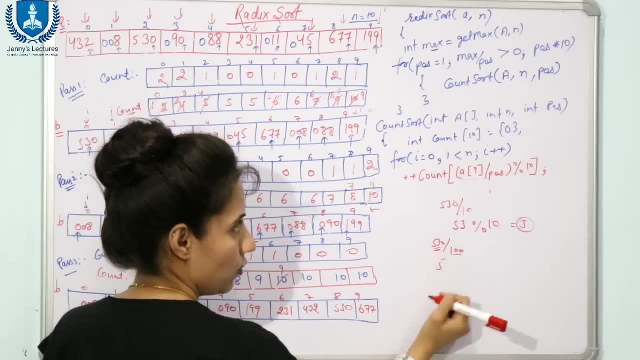 this 530. so in third pass we are going to deal with this. 5 only 530 divide by post value in third pass is 100. so now the this divided by 100 is what? 5 only, 5 more 10 is 5 only. so we are going. 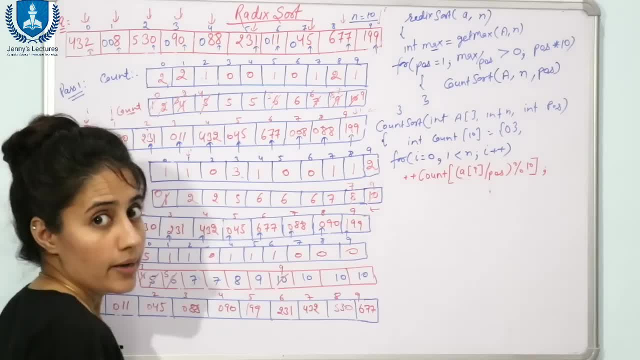 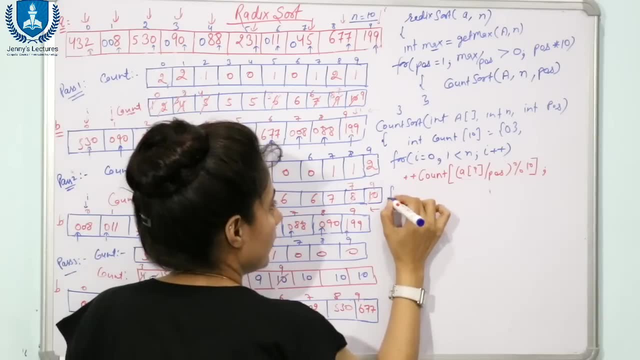 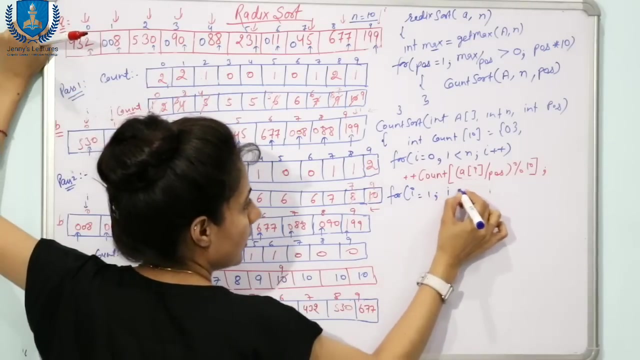 to deal this 5 only. so this is the exact logic. so now next for loop would be for this array to update this count array to reflect the actual position. so next for loop would be: we are going to start this from 1, because first value would be, as it is, 1 till i, less than equal to k and 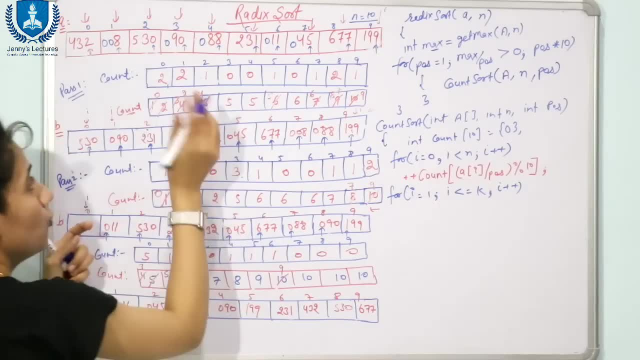 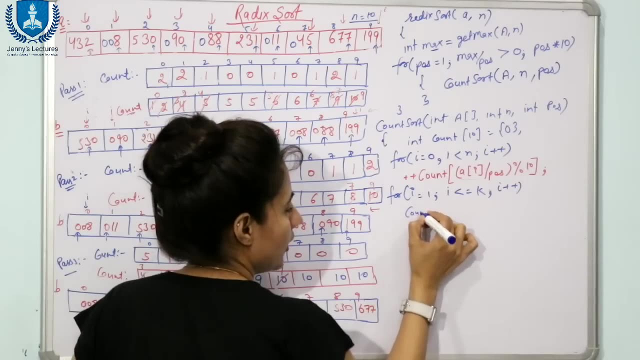 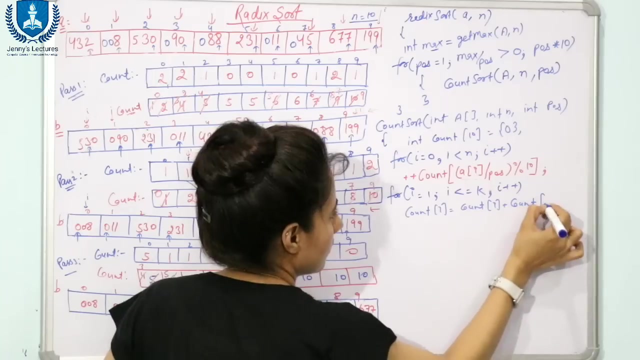 i plus plus. now here what you will write: we will simply add this plus this, next plus previous. so that is very simple. so simply, we are going to write: count of: i is equal to same count, i plus count, i minus 1. this is the same we have discussed in the count sort. now third would be to build. 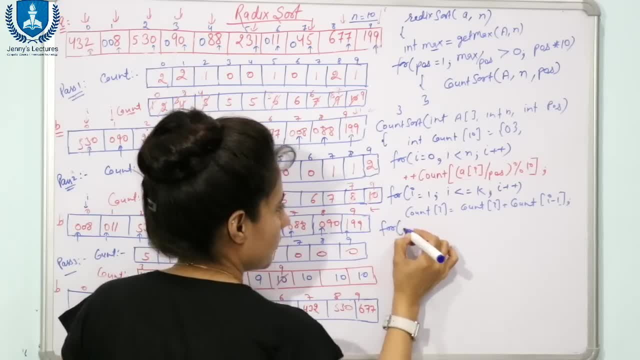 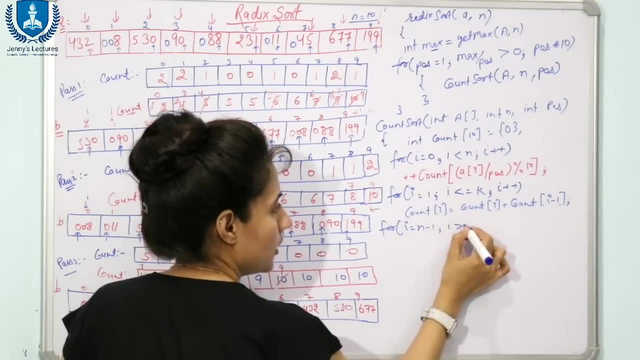 this array. now, third for loop. we are going to start this for loop from here. we are going to scan this array from right to left. so i would be n minus 1, i would be greater than equal to 0 and i minus minus. so what we have done in this case, 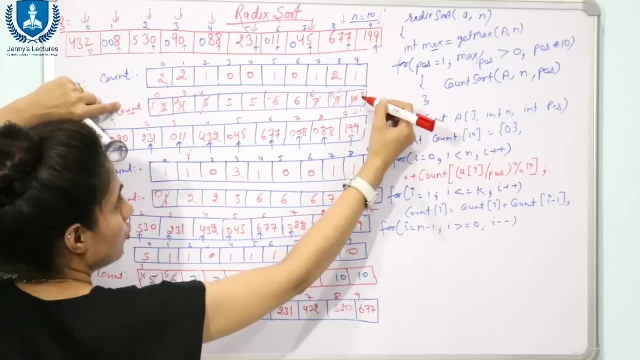 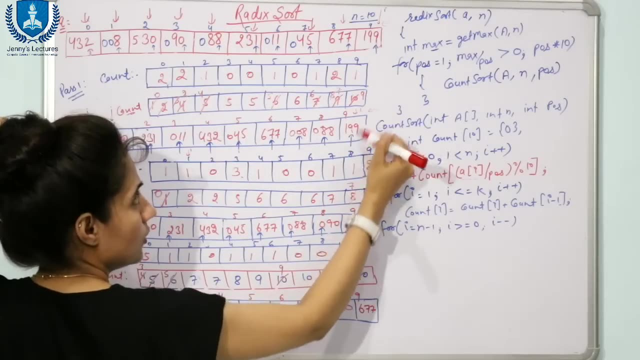 we have just taken a count of i and we are going to write: count of i is equal to k and i plus count nine. go to the index. nine is count sort decrement, this counter value, and in the output array b, at this index nine, we stored this value. fine, so this value would be stored where. so this value? 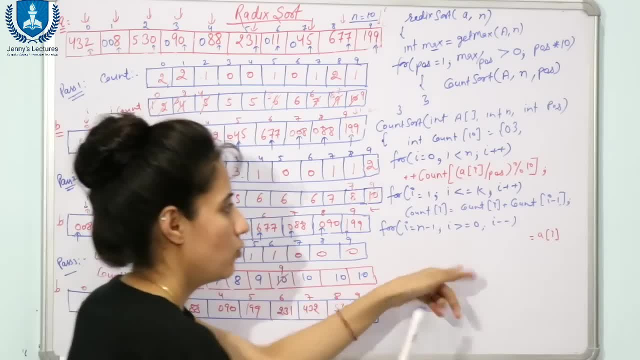 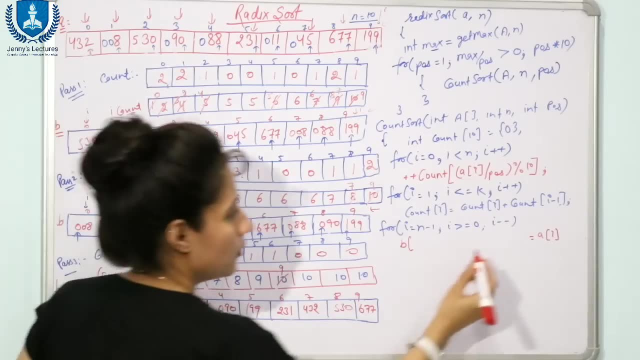 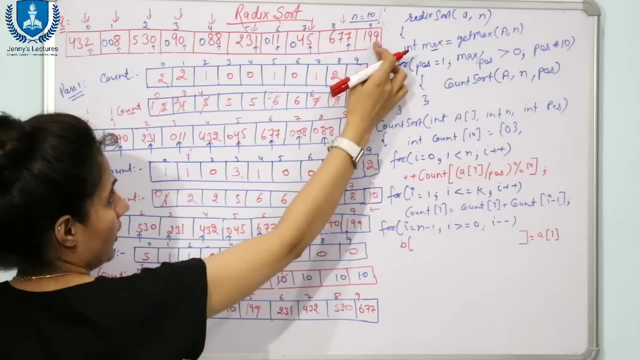 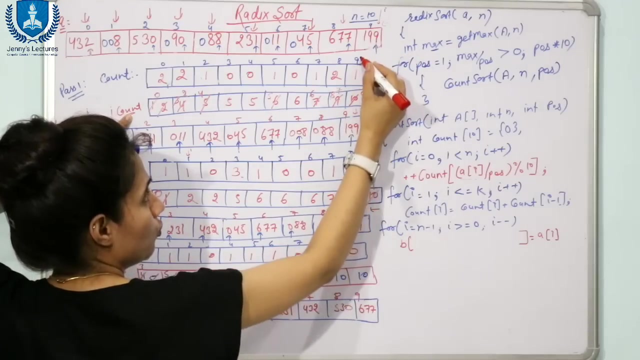 that is a of. i would be stored where you are going to write down that thing here, obviously in the b array. but index would be what? so now see what you will write here: how to calculate this index that is nine for 199, using this count array. in count array this value is nine. we are going to 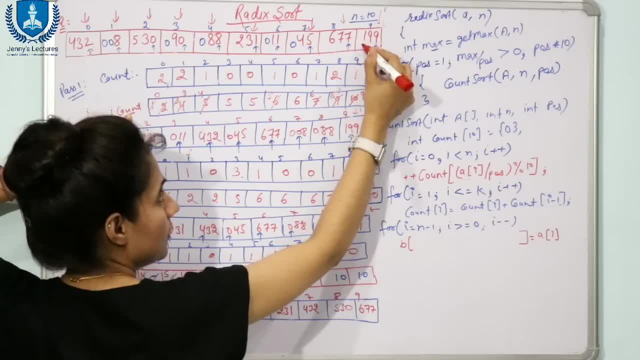 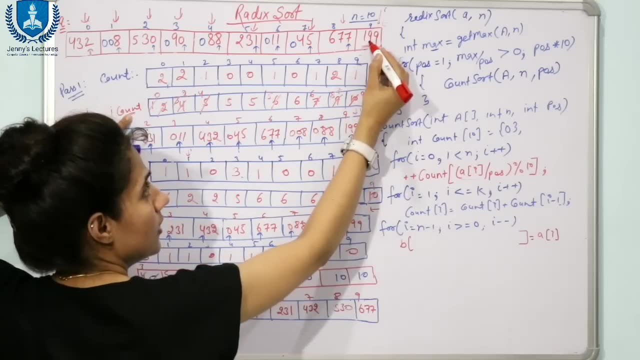 check the same index. fine, so first of all, in out of this, out of a of i, you have to find out this nine and you can find. in second pass, you will deal with this nine, and in third pass, you will deal with this one. how to find out these particular digits using this logic only. 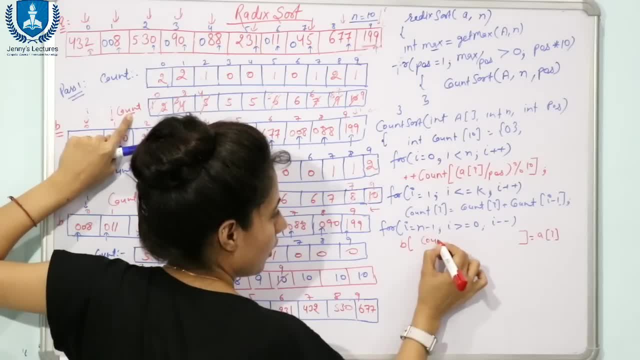 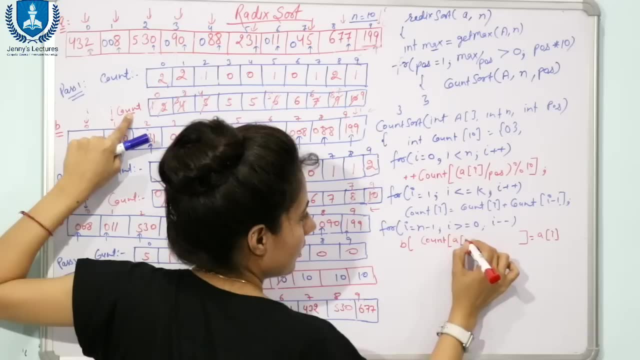 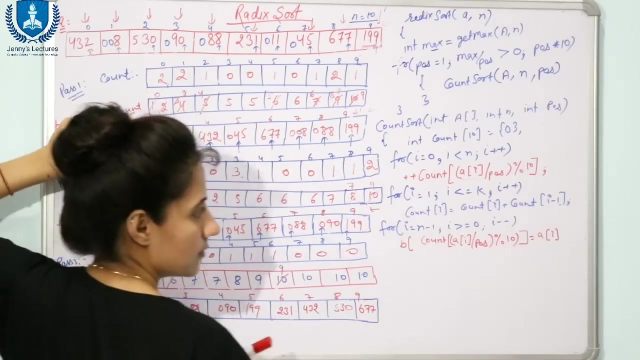 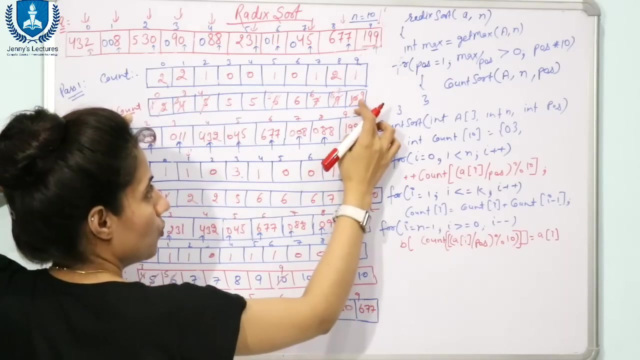 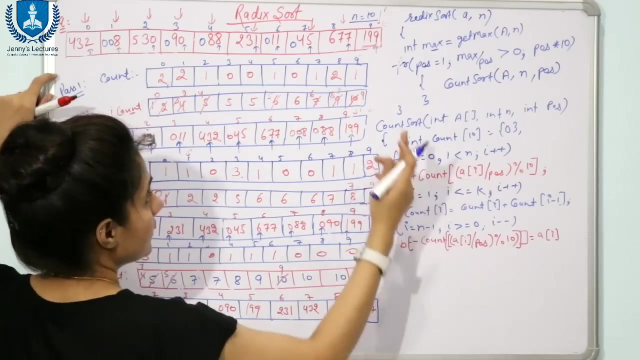 we have already discussed, so now what you will do count and index, how you will calculate same a of i divide by pos mode 10. fine, this is how we are going to calculate the index of count. and then you will do index, rible this, this value minus minus, then you will do minus, minus. so you can. so you can take one example: see: 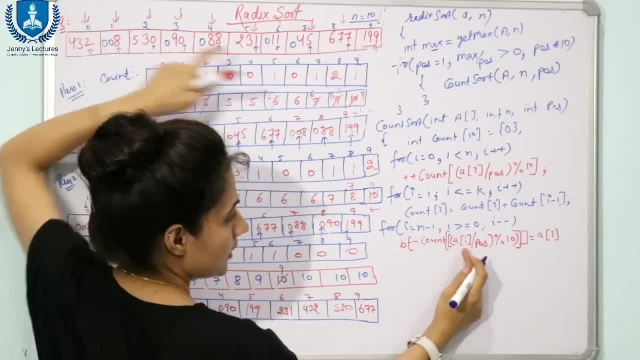 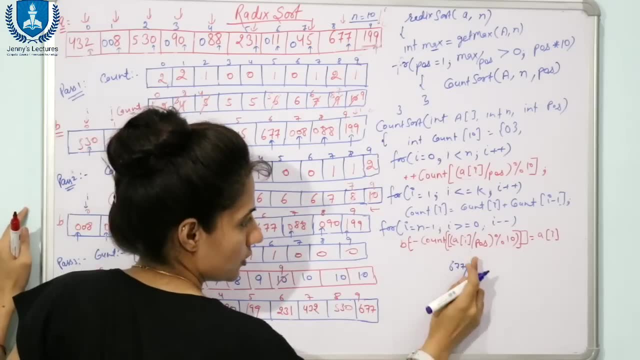 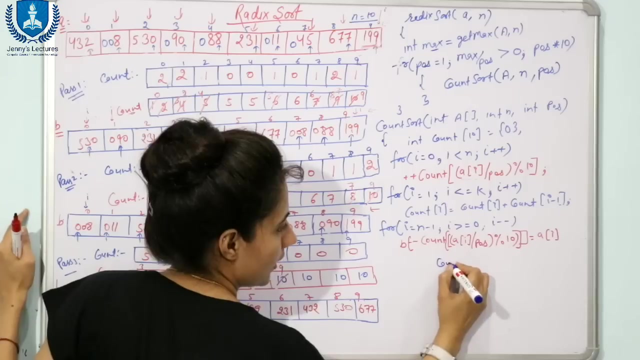 let us take the 677. a of i is 677. 677 divide by in first pass, this pos value is only 1. so 677 divide by 1, that is 677 mod 10. mod 10 means 7 only. so here you will write count 7. fine, now. 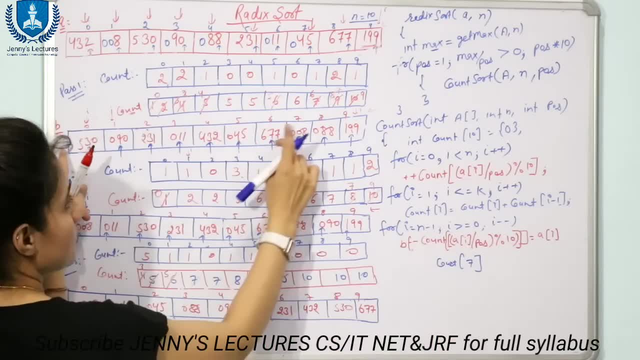 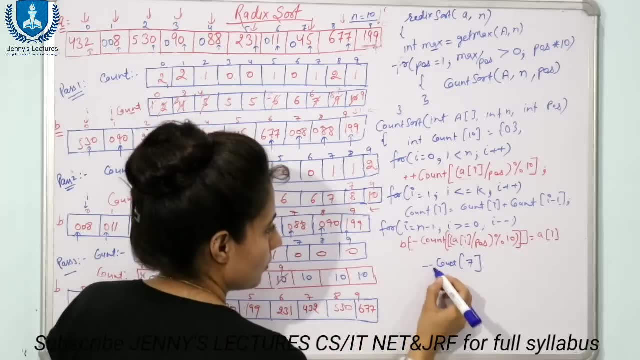 count 7 minus minus. go to the index 7 here. go to the index 7. here we have 7, but minus minus. then 6 minus minus. here we have b. after minus minus it becomes 6. so at b of 6 you are going. 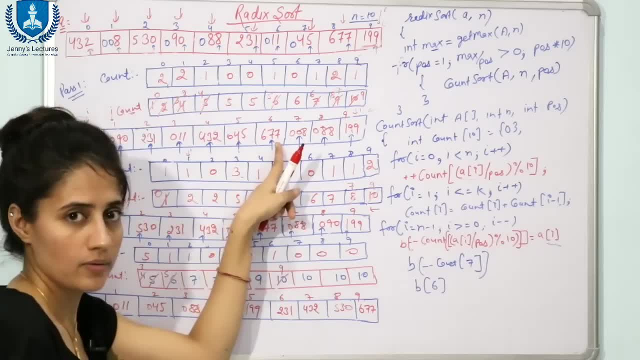 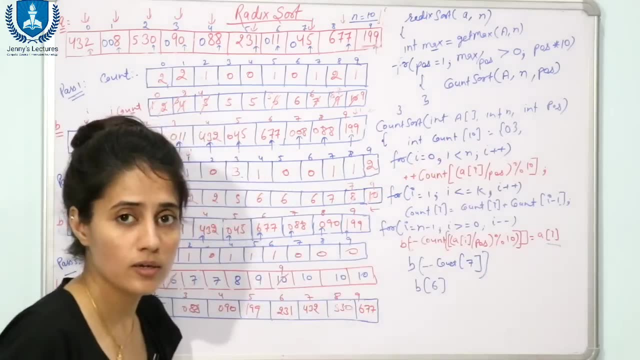 to store 677. you are going to store a of i. this is how this logic will work. in second pass, same the pos value would be passed from here. that is n only so you can trace out the complete pos value from here. that is n only so you can trace out the complete pos value from here. that is n. 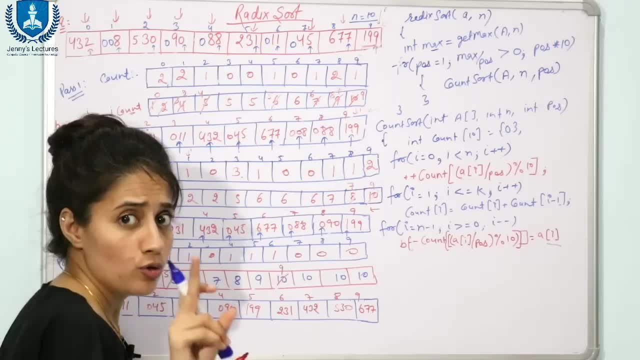 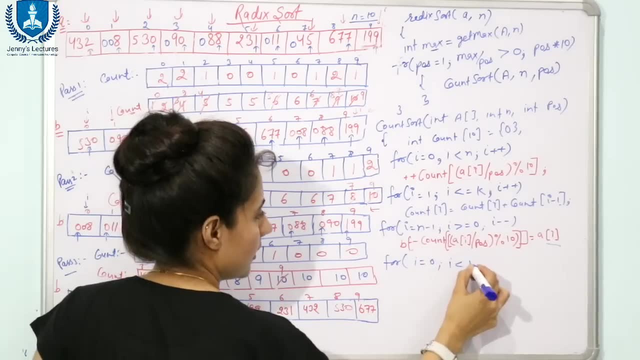 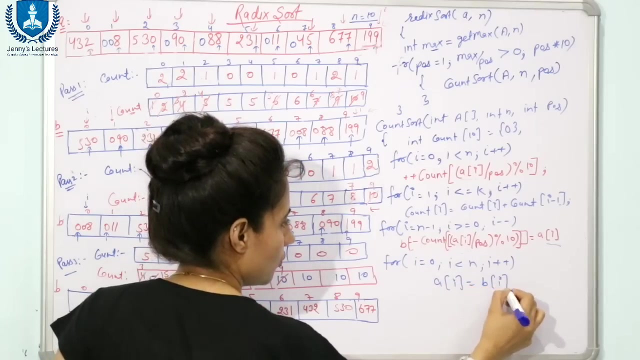 code with the help of this example. and now, simply, the fourth loop would be what to copy the area of this to this? so one for loop. i is equal to from 0, i less than n and i plus plus, and this would be just copy the elements of b array into a array. see, this is not the complete. 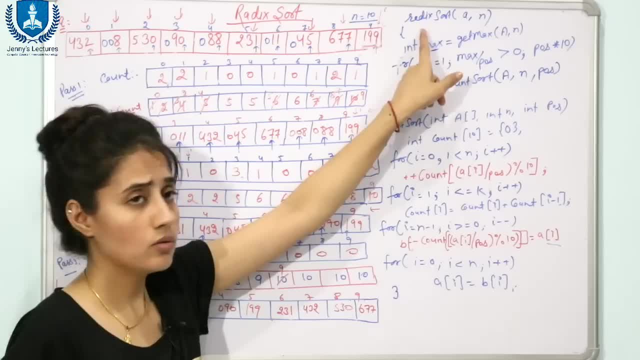 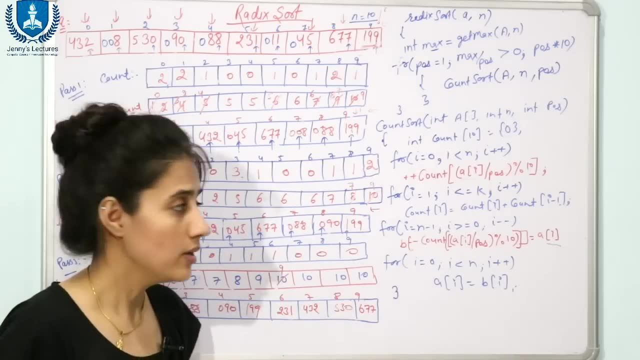 program you are going to write down the main function. in that main function you will call: call this radix sort and you are also going to write down the code for this getmax function. fine, but this is the main logic. you can trace out this logic with this example. 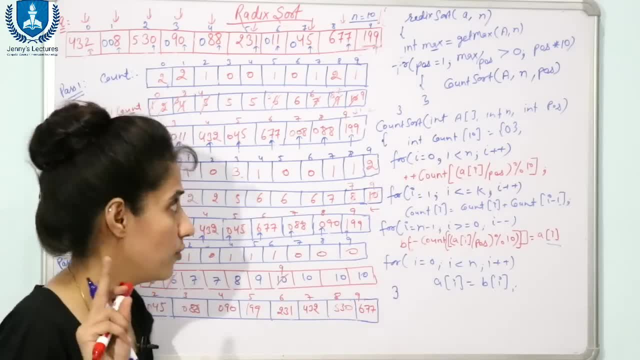 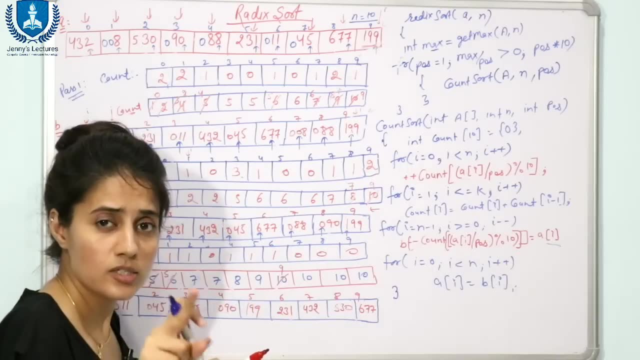 for each pass. i am not going to trace out this one because the video would be very lengthy. now i am going to discuss the time complexity see time complexity for this count sort is what we have discussed in that video when we were discussing counting. so that is order of n plus k. 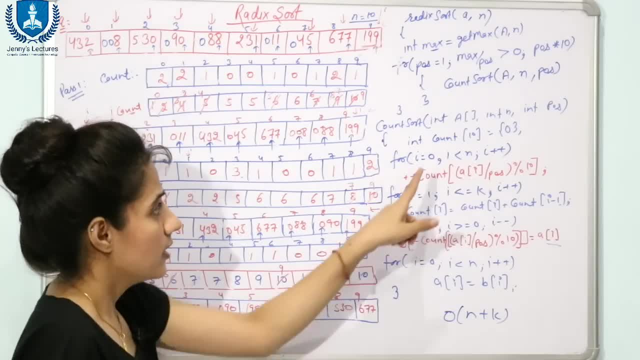 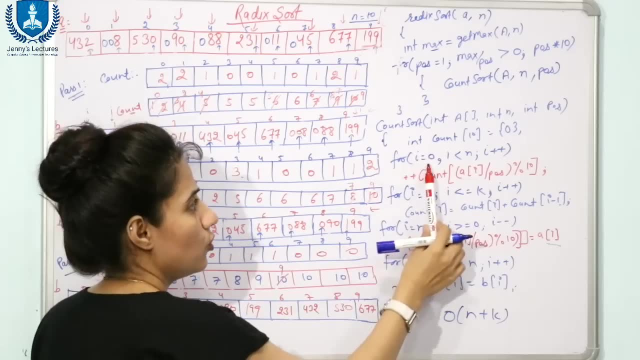 why n plus k? because see how many four loops, four four loops would be there, how many times the calculation would be there within these four loops. so this is the order of n plus k. so this is the order of n plus k. so in the case of four loops, this four loop would be. 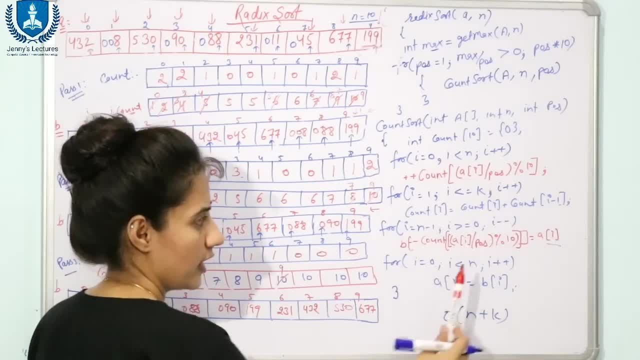 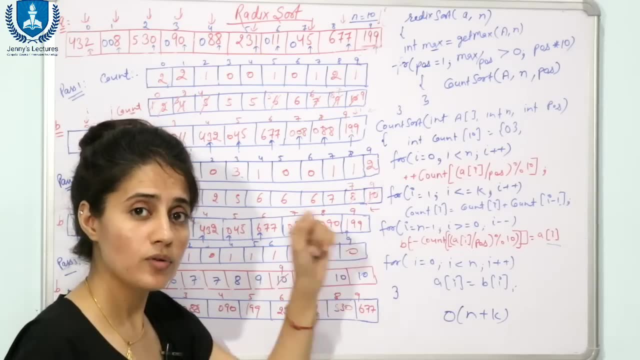 from 0 to n. that is n times. this is k times. this is n times, this is n times. so 3, n plus k, that is n plus k and how many times this counts. so it would be called the number of digits in the max data here. three times it would be called so you can write time complexity.